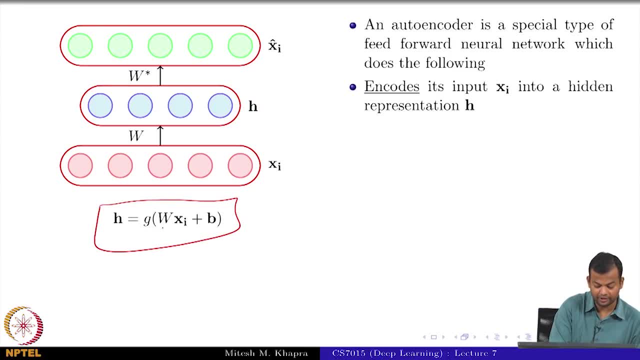 function to do this. So this is what the encoder function does. it first does a linear transformation. W is a matrix and X, i is a vector, and you again have the bias B as a vector, right? So let us look at these dimensions, right? So let us try to fix some dimensions. So suppose, 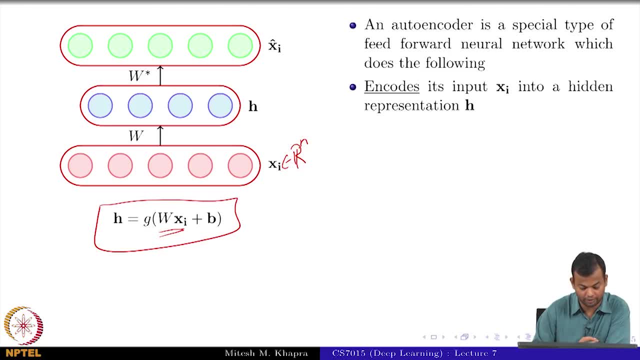 X, i belongs to R in. that is what we have been considering throughout the course so far. and let us say H belongs to R d. ok, So it is a d dimensional representation. So in that case, what would W be? Yeah, So W would be R n cross or other d cross n right, So it? 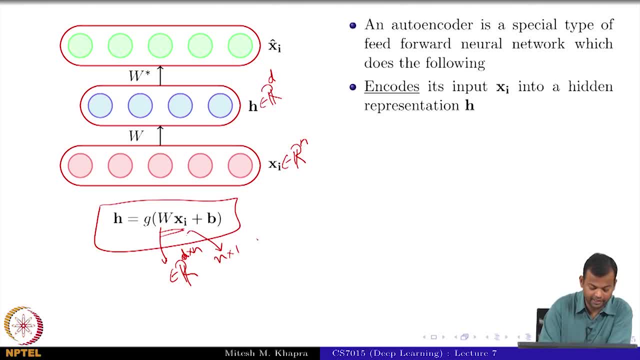 will multiply with a n cross 1 vector, which is X- i, and give you a d cross 1 output right, and similarly the B would also be d cross 1, and then on top of that you have this nonlinearity g, which will be operating at L- i. 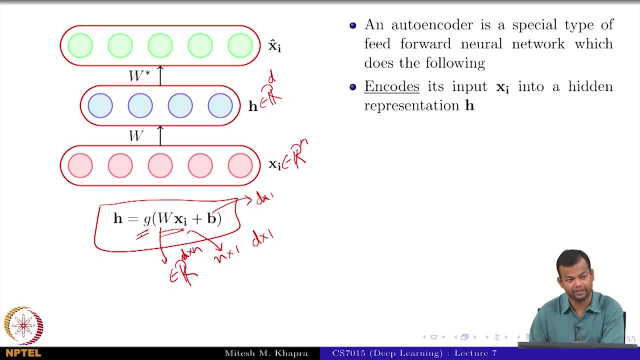 So element wise, just as we had seen earlier. So it could be any of the sigmoid functions, the logistic or tan H, and so on. So the end result is you have taken an input X- i and encode it into a hidden represent H by using a linear transformation first and then a nonlinear. 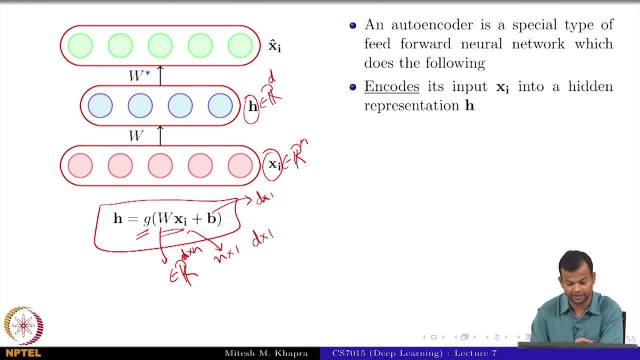 transformation, right, So I refer to W X plus B as a linear transformation, because it is a matrix multiplication. Now, once you have constructed this hidden representation, the job of the decoder, or the latter half of the feed forward neural network, which is this half, 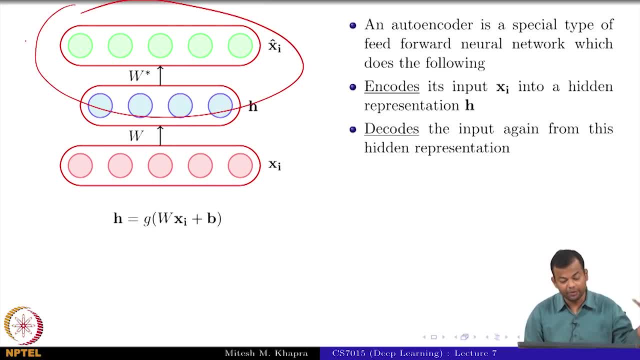 So what we are going to do is to take this encoded representation and then try to reconstruct X again from it. ok, So again, let us first look at the equation. So this is the equation for the decoder, where again, you first take the hidden representation, do a linear transformation. 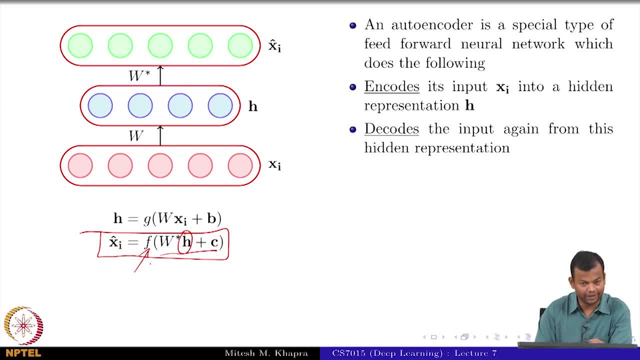 and then you again have some function or nonlinearity on top of it, right? So we will see what this function can be, So we will refer to it as F. for now we will not say whether this is sigmoid or linear or what kind of a function it is. we will come back to it later. 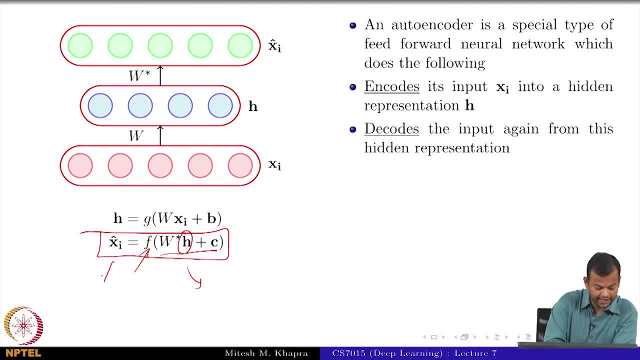 So now let us again look at these dimensions. So what is X i? X i is again R n and your H was R d. So you have to go from a d dimensional input to an n dimensional output. So again, 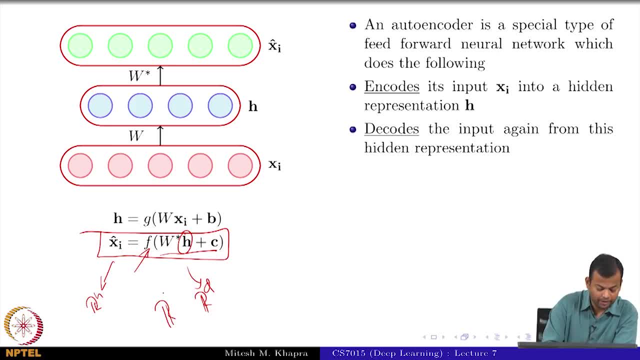 your W star is going to be R d cross, sorry, R n cross d, So it will multiply with a d cross 1 vector and give you an n cross 1 output, right, and that will pass through some function And it will give you X i hat, which is a reconstruction of X i ok. 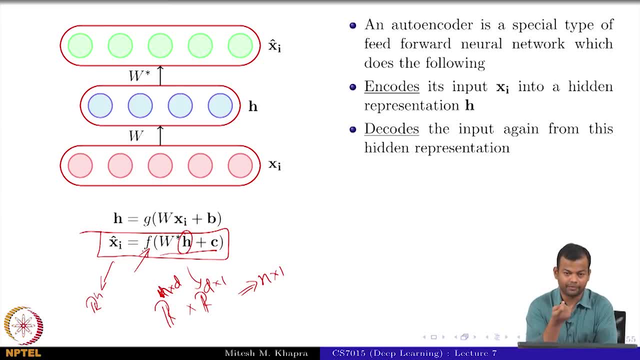 So why are we trying to do this? right, we took an input X i, we computed its hidden representation by doing some non-linear and linear transformation, And then again we are trying to reconstruct X i hat. So why are we trying to do this? 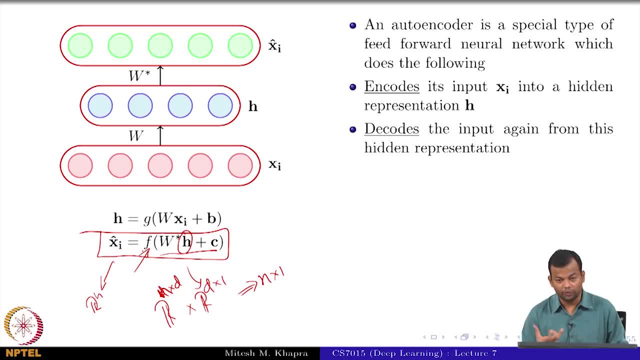 so reason we are doing this is that we want to learn what are the most important aspects or most important characteristics of the input data X i right. So if you compute representation H, which is presumably smaller than your original input data, and from that 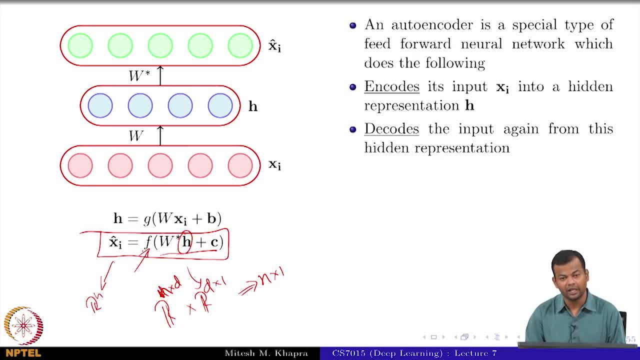 hidden representation. if you are able to reconstruct x- i- right, then that would mean that this hidden representation captures everything that is required, or everything that is, yeah, everything that is required to reconstruct x i from x i from the original input, right? So the model will be trained to minimize the difference between x i and x i hat. So 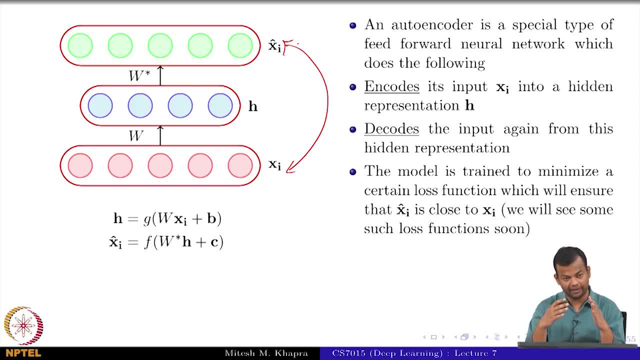 you want to make sure that, after passing through this bottleneck, which is the hidden representation, you are able to reconstruct x, i, and the reconstructed output is very close to the original input, right? So can you see an analogy with PCA, where you are trying to find this hidden representation? 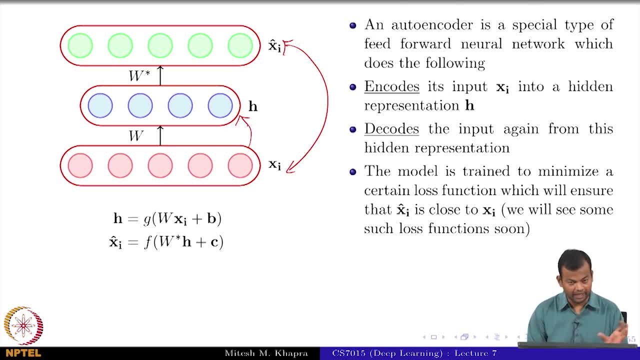 or this most important elements of the original input x i. So there we had used this linear transformation, where we had taken the original input x and transformed it to a new basis and we had used that, That basis, for representing the original input right. So something similar is happening. 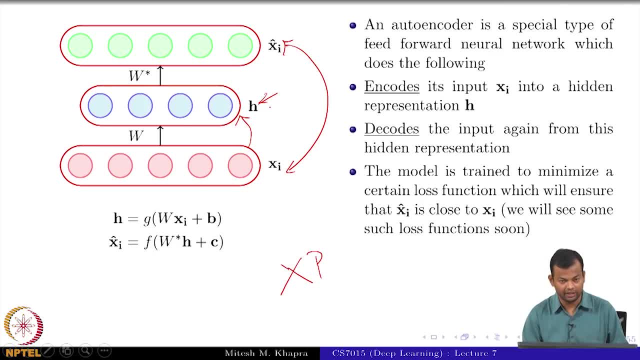 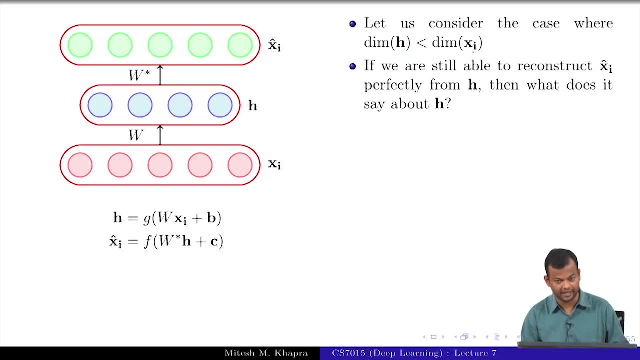 here we are using this hidden representation, H, to represent our original input. Now let us consider a few cases. the first case is when the dimension of H is less than the dimension of x. i In this case, as I was trying to say earlier, if we are still able, 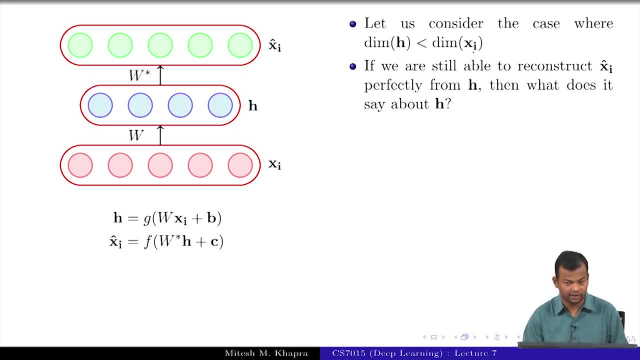 to reconstruct x i hat perfectly from H. then what does it say about H? It tells us that H is a loss. free encoding of x i. it captures all the important characteristics of x i. right, just repeating what I had said on the previous slide. And now you can see an analogy with PCA, because H has all the important characteristics required. 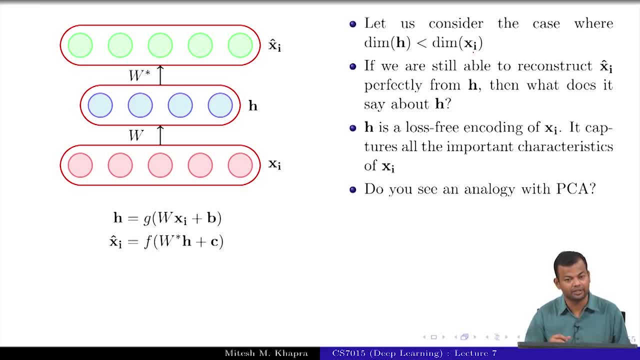 from the original input data, So it has probably got rid of all the noise or all the low variance dimensions or the correlated dimensions and so on. This is just the compact representation, which is as good as the original representation, and from there you can reconstruct the original. 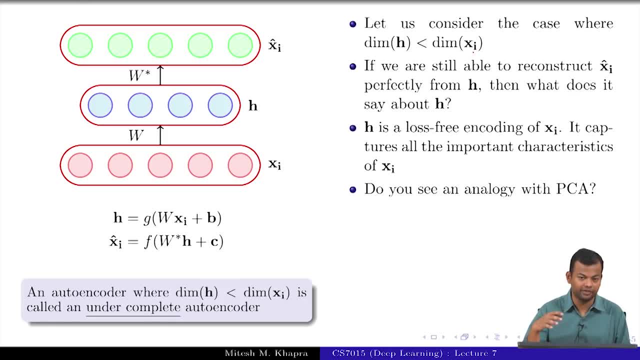 representation And such an autoencoder where the dimension of the hidden representation is less than the dimension of your original input. So this is a very important point. So I am looking. maybe while I am having a formal conversation I want to drive around. 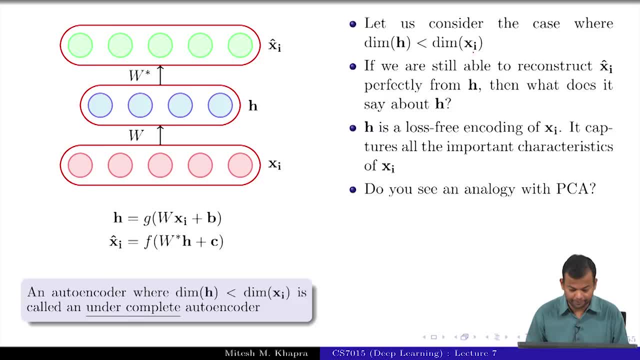 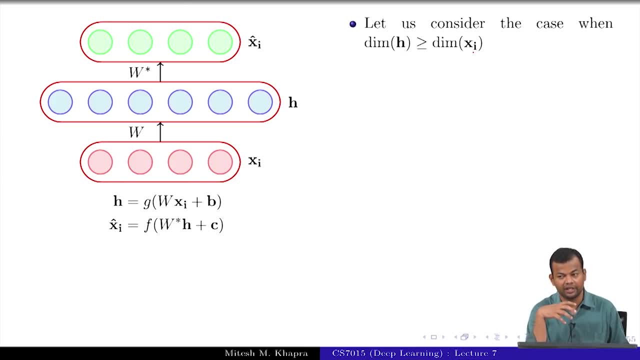 the subject. So what these two commands mean is that the dimension of H is less than the dimension of the original input. right By that I am hastaing to understand why here same example. So this is the dimension of H, apart of H dot, H itself. or H. low number H is less than H. hat right. So H m H on top又. mes you are coming up is 1 0 2, 0. right Now, we are basically trying to cross out these two terms, So let us. celebrate at least one component: the dimension of H. H is less than the dimension of H, empty cell 1, so we are considering here that H puede ser 1, 2, 1, h are considered like a Yankee square, or 1, 2, 3, 4.. In this scenario we are considering, say, 2, 4, 5, 8, 7, 8, 7, 8, 5 properties. 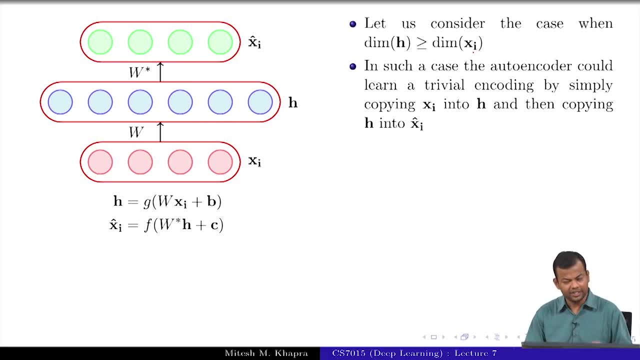 is greater than the dimension of the original input, right? So now, in such a case, the auto encoder could learn a very trivial encoding by simply copying x i into h and then copying h into x i, right? So think of this from a compression point of view, right? So now suppose, 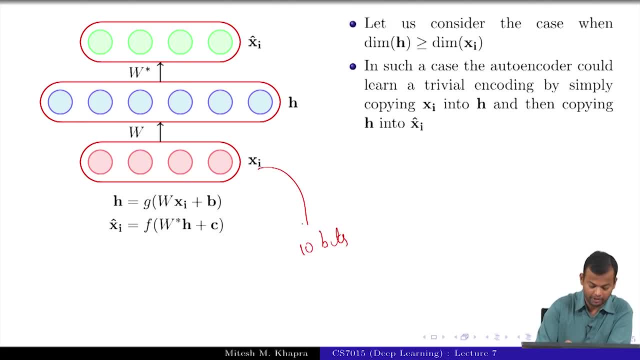 you have 10 bits, initially right, and then you want to somehow compress it and store it only in 4 bits. And now this 4 bits should be such that it captures everything that was there in the original 10 bits, because you would want to reconstruct the original input. 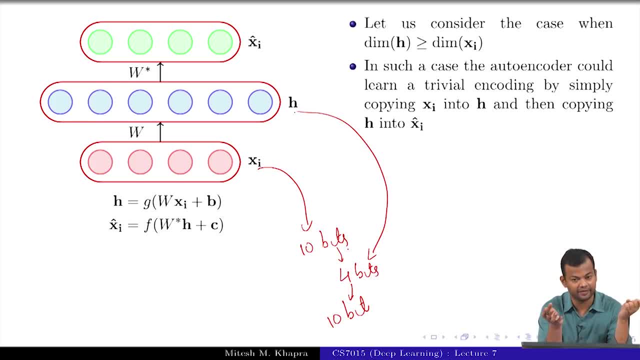 again, right? So this is what we do typically when we compress any of our files. right, We have a larger file, we compress into smaller information, while making sure that everything important is there, So that whenever I want to recover it, I can just recover it from there. 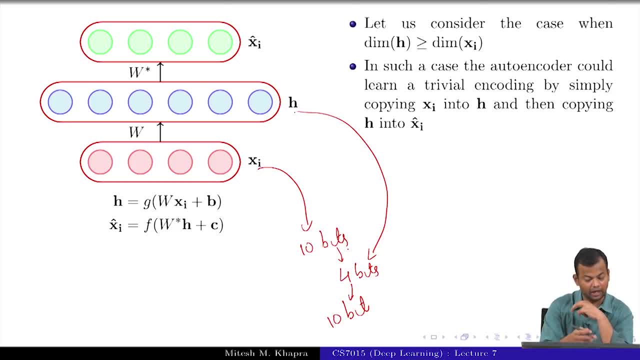 right. So this is definitely a hard task. but now what I am doing in this auto encoder is that I had 10 bits- I am actually giving it more bits now because the dimension of h is greater than the dimension of h Of the input- and then from these 16 bits I want to reconstruct the 10 bits Now. this: 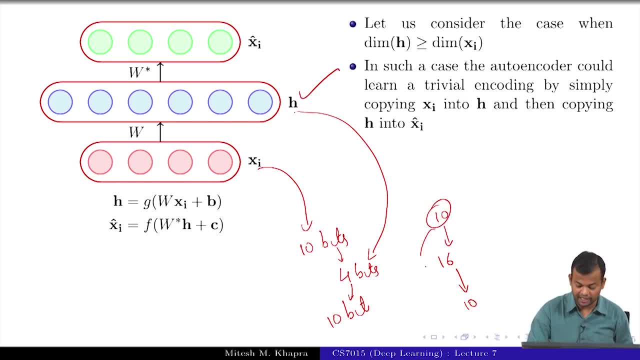 is a very trivial task, right? because all I could do is copy these 10 bits into the first 10 bits here, leave the remaining 6 blank and then from those 10 bits just reconstruct the input. that is very, very trivial If you give me more storage and what I originally needed. 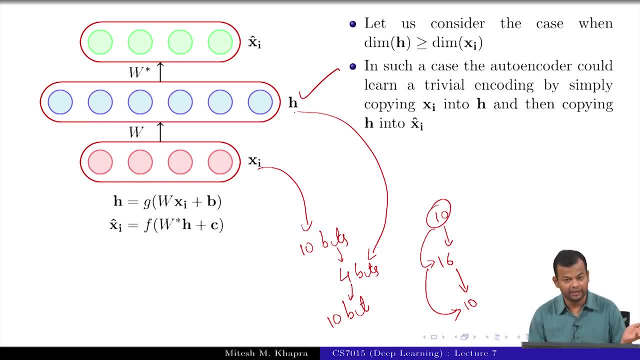 then definitely, I can easily reconstruct it right. So this looks very trivial and this is what it could do, right? just copy the input to the first n bits, Right? So this was n and this was d, and we are looking at the case where d is greater than n. So 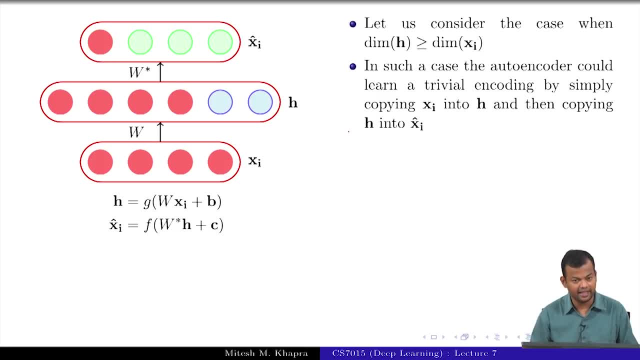 it could just copy the input to the first n bits and then just take it back to the output. just as I said, in the case of you have 10 bits, 16 bits and then again 10 bits. it is very trivial to do this. So such an identity encoding is useless because you are just not. 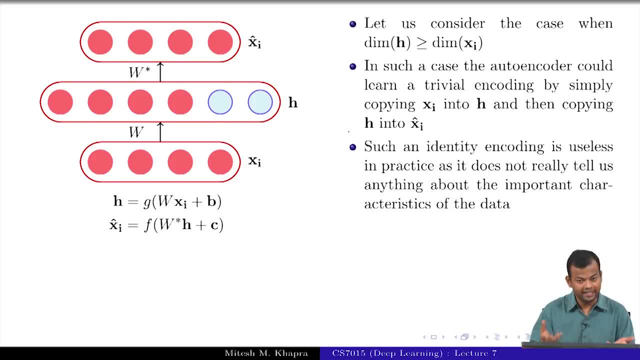 running any important characteristics of the data. your h is almost the same as x i. it also has all the useless information that x i had. In fact, it has slightly more because it has these blank units, Right? So it has these blank units also, but this is not really useful, right? why would you want? 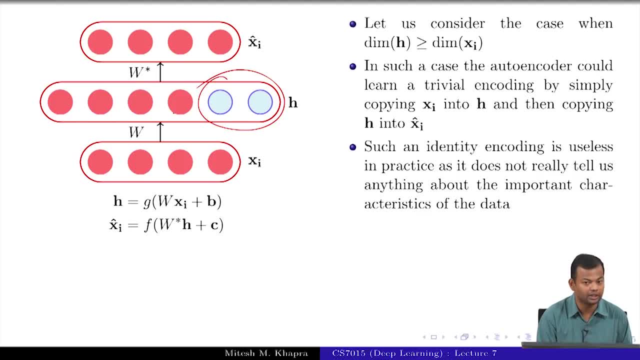 to actually learn such a hidden representation, right? So it is not clear why would you want to do that? So we will take a look at it. we will come back to why this is important. So such an autoencoder is known as an over complete autoencoder because it has the hidden representation has. 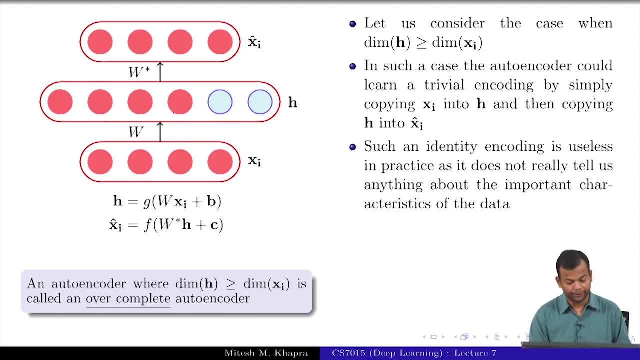 more number of neurons as compared to the original input. Now let us look at a case where this would actually be important, right? So this is a very rough intuition for why you would want an over complete autoencoder, correct? So let us consider the case where you have as input one of the features that you are 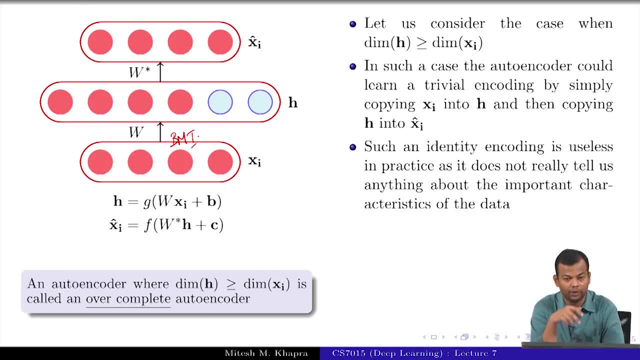 looking as BMI. So suppose you are trying to find out whether the person is likely to get a certain disease or not, right, whether he would have a heart attack, or whether you would have a diabetic, would have diabetes, and so on, and we are looking at various parameters. or various medical parameters of that person. 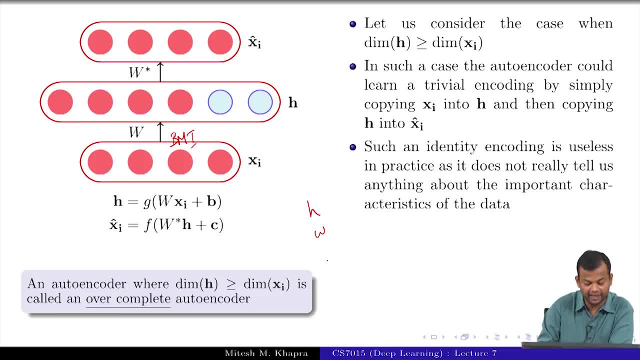 of that person, and one of them could be height, one of them could be weight and one of them could be BMI. Now, for whatever reason, you have not computed the height and weight and you only looked at the BMI. So now what is happened in your input? and all of you know that BMI is actually body- 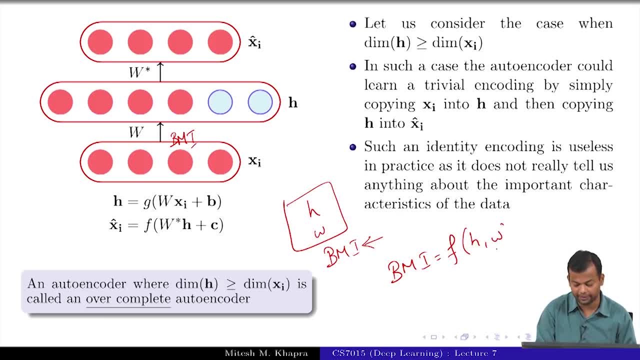 mass index, which is a function of the height and the weight. So now what is happened is that in your original input there was already this compact the. your feature space was already compact because you would actually looked at- you should have actually looked at- both the features height and weight, but for some reason you 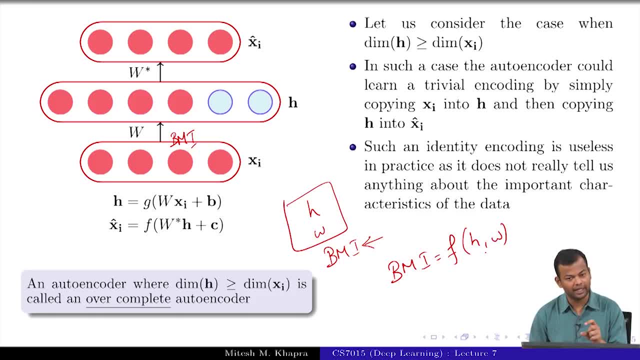 have only computed BMI, And you could think of various, some other correlated features which are functions of many other features, but you do not look at all those features and just this final function of those features, right So now, in that case, if suppose your prediction is that this person has, or has, a high likelihood, 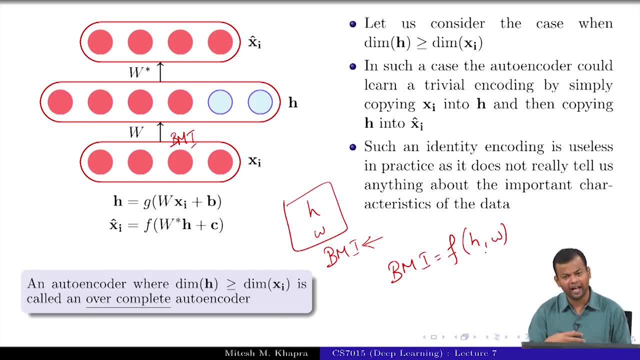 of being of high likelihood of having diabetes some at some point in his life. then you would want to know Whether it was the height or whether it was the weight which was responsible for this. So in your original input the features are actually entangled and you would like to disentangle. 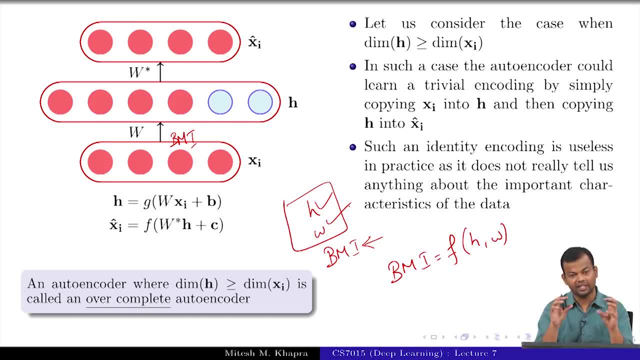 them right. So you would want to go from this smaller feature space to a larger feature space where some of these entangled features get disentangled. So in those cases we need to search an over complete autoencoder. However, the problem still remains that there is no reason why the machine should actually 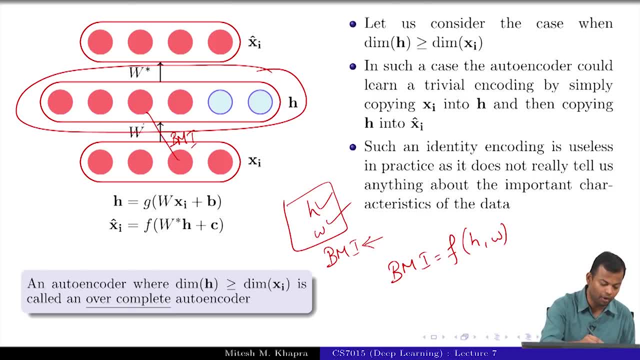 learn to disentangle this features. it could still just simply copy the BMI here And then copy it back here, right? So that is why, when you are dealing with over complete autoencoders, you will have to do something special to prevent these kind of identity encodings where you just take 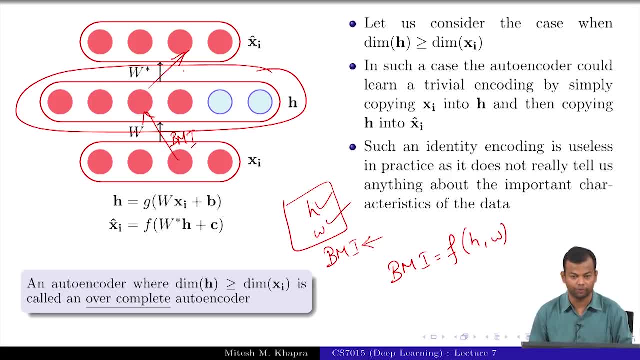 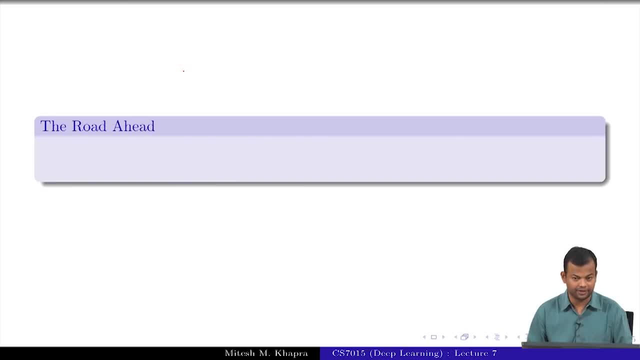 the input and copy it to the hidden layer and then copy it back to the output. So we will look at what kind of special treatment you need to do to prevent these kind of identity representations. ok, Here is the road ahead. So first we will talk about the choice of FXI NG. 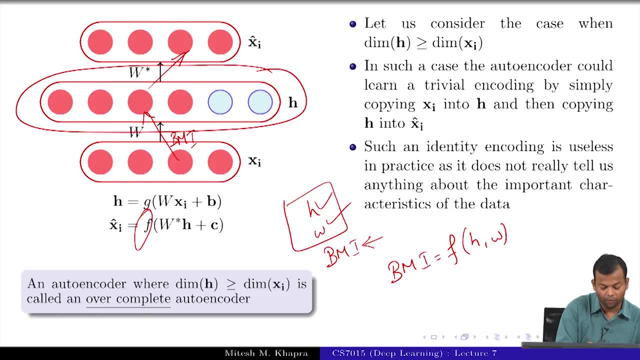 So we did not say anything about what these functions F and G have to be. So we will talk about those and then we will talk about the loss function. So I have just told you so far that we will train this model in a way that X i is very. 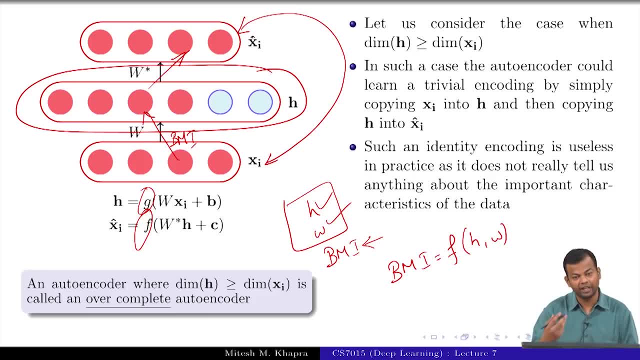 close to X i hat right, And I have argued that if we are able to actually achieve that, that X i hat is the same as X i, in which case presumably the loss would be 0.. That means our hidden representation has captured all the important characteristics of the original. 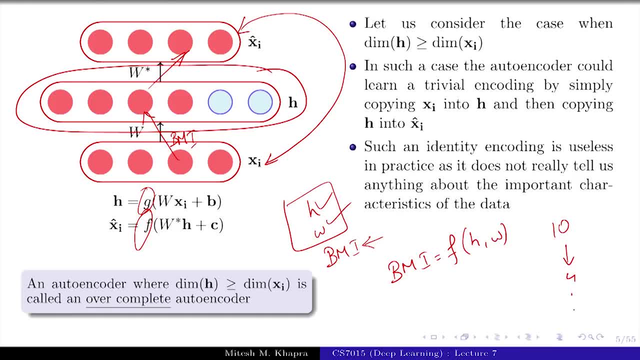 data Same as in the analogy of 10 bits to 4 bits to again 10 bits. right, If I am able to reconstruct this without any error, that means loss is 0. then these 4 bits, or the hidden representation of my original X, was actually able to capture everything. 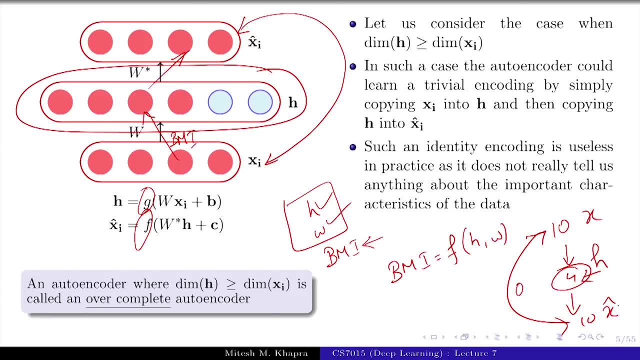 that was important in X, So that it can reconstruct X again, as X i hat, without losing any information, right? So that is the loss function that we would want. Now, what is the actual mathematical formulation for this loss function? that is what we will. 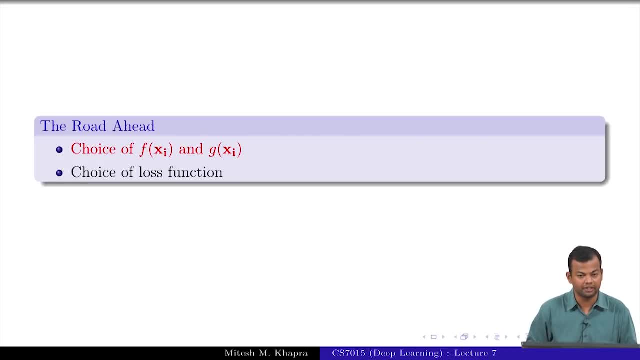 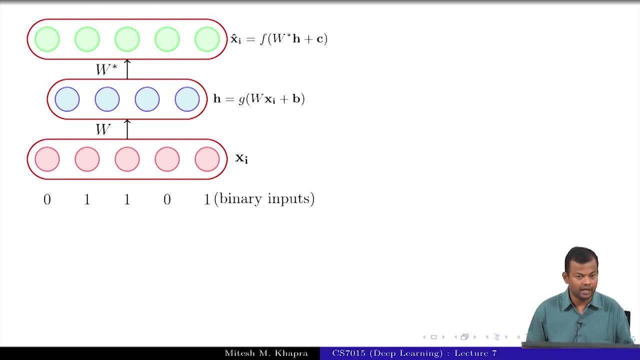 see next. ok, So first let us start with the choice of F and G. So we will consider 2 case, 2 cases: 1 case when your inputs are binary and the second case when your inputs are actually real numbers, right? So first we look at the binary case. ok, 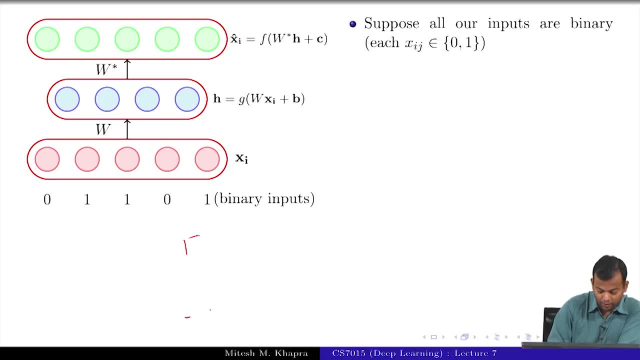 So now just some notation clarification. So remember, our original data was this: matrix X, which was m cross n. that means you had X 1, X 2 up to X m, And each of these was R n. right So now, when I am referring to the entire row or entire data instance, I will use bold. 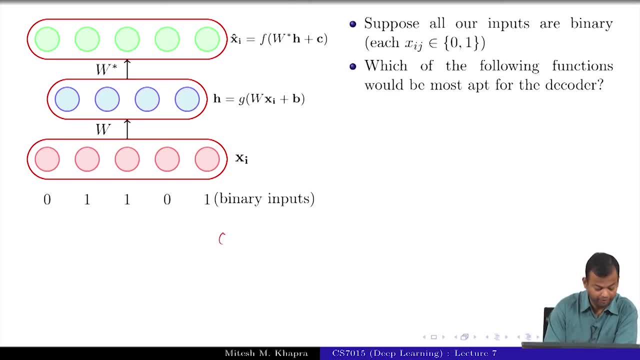 X i, as I have circle here and I want to refer to 1 of the elements of this guy, then I will use this notation: X i j, same as what I have written here. So what I am saying is that each of these X i j's actually is a binary variable. ok. 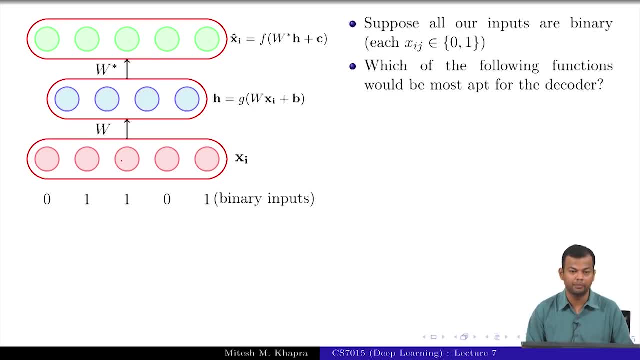 Now which of the following functions would be most appropriate? I have some studies So it is not compulsory. What are the steps appropriate for the decoder? So remember your input was binary. that means your output also has to be binary. you do not want to produce numbers arbitrary large, belonging to any or 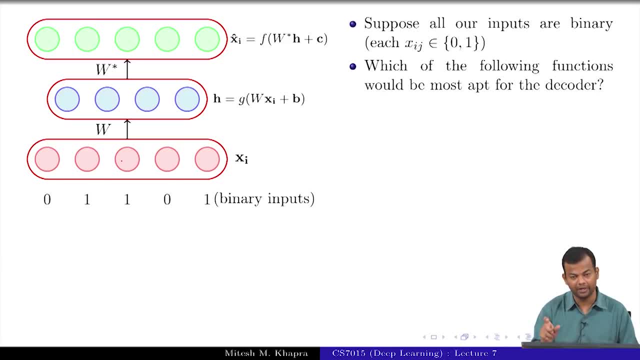 you do not want to produce any real number, you want to produce numbers which lie between 0 to 1.. So, in such a case, what would be an appropriate loss function or, sorry, what would be an appropriate function for the decoder? So remember, I am asking you what would f. 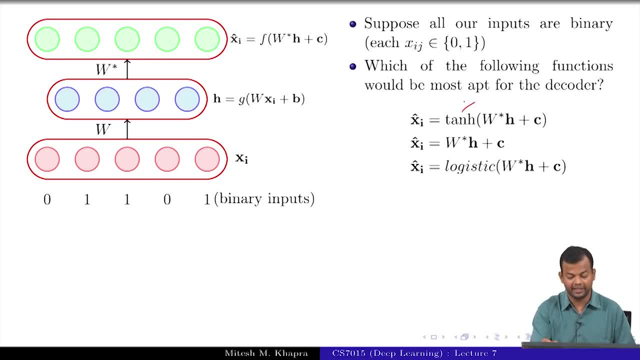 be. So I am giving you three choices. it should be tan h, or just a linear decoder, or a logistic function. which of these would be most appropriate? logistic? why would that be? because it will make sure that your outputs are between 0 to 1. tan h would give you outputs between 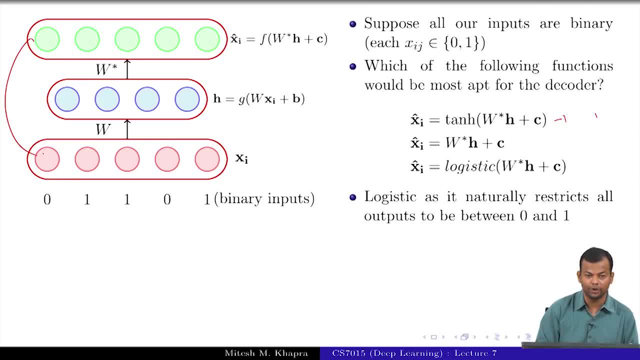 minus 1 to 1, but you do not want that because your inputs were between 0 to 1.. So when you are reconstructing, obviously you want outputs between 0 to 1, you do not want minus 1 to 1, and linear, of course, can give you any real number, and which is not what you. 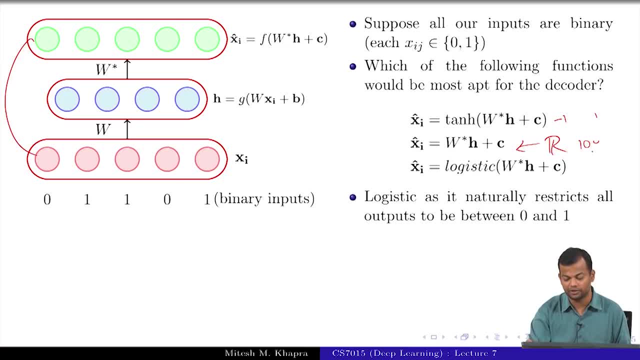 want right? So if you produce any arbitrary real number like 100 and so on, your loss is going to be very high, because your inputs were just 0 to 1 and you are producing these arbitrary real numbers which are very different from what your input was. ok, So in this case, the 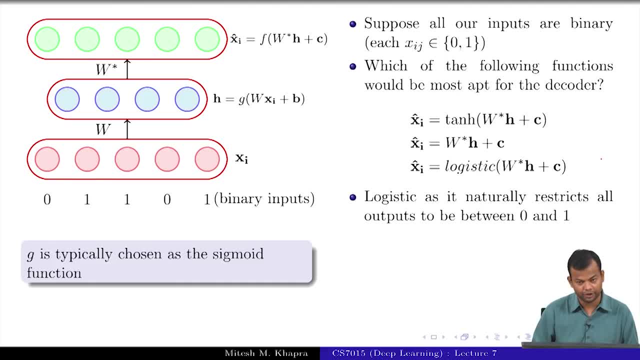 logistic function makes the most appropriate choice and g is typically. that means the encoder function is typically again chosen as a sigmoid function. So it could either be the logistic function or the tan h function. right, So there is a. you could choose any of these as the encoder function. ok, 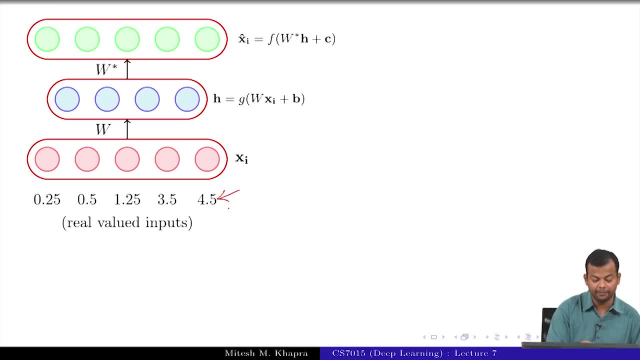 Now let us consider the other case, where your inputs are real valued. that means when you reconstruct something, you should again produce real values. that means your function f should take whatever is the input given to it and map it to some real numbers. right? So that is what we want from this function f. earlier in the binary case we wanted it. 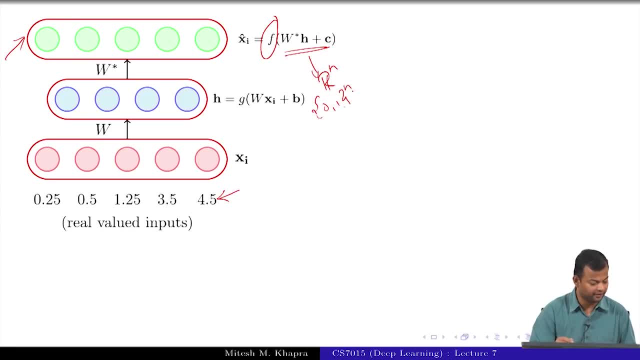 to map it to binary numbers, right? So that is the difference that we have now. So, in this case, which of the following would be appropriate? The second one, right, because tan h does not make sense, because it will just produce minus 1 to 1, but you want to. 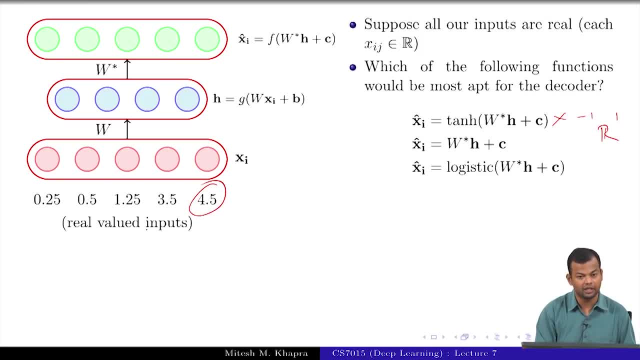 produce any possible real number, because some of these are actually higher than 1, greater than 1.. Linear would be fine because it will produce any real number. logistic is again not fine because it will produce numbers between 0 to 1. ok, So the logistic and tan h, as I said, would clamp the output to certain ranges, So that 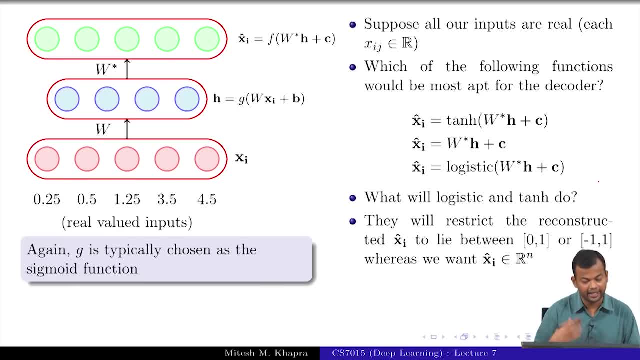 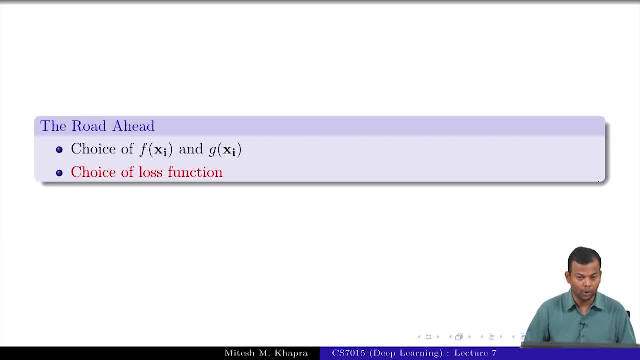 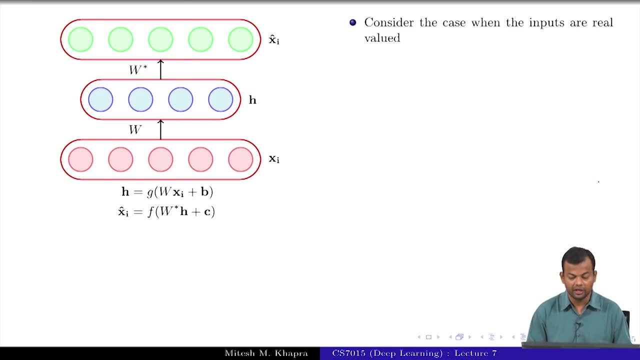 is not appropriate. hence you should choose the linear function. and again, in this case also, d is typically chosen as the sigmoid function, right, ok. So the next thing that we look at is the choice of the loss function. ok, and again, we will consider both the cases where the case first case is the inputs are real valued and 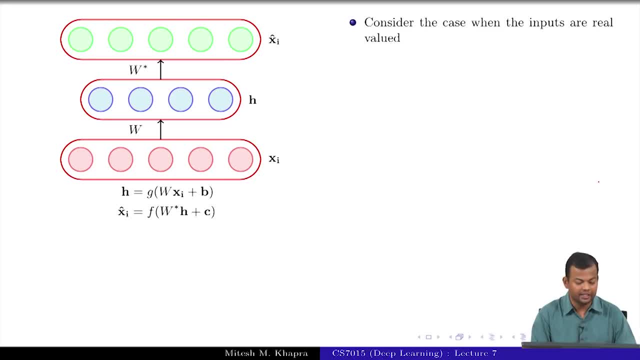 the second case is when the inputs are binary. ok, So let us look at the real case first. So here the objective of the autoencoder is to reconstruct x i hat to be as close to x i as possible. Now we have actually seen this before, So something similar before. 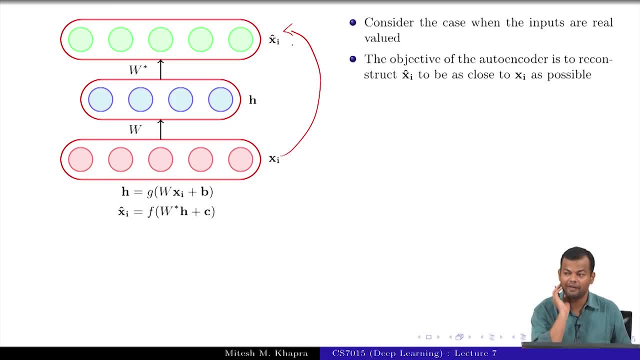 when we were talking about regression. So now you want to produce real valued outputs and they should match your real valued inputs. So what is an appropriate loss function that you can choose? The squared error loss function, right. So what does this actually capture? 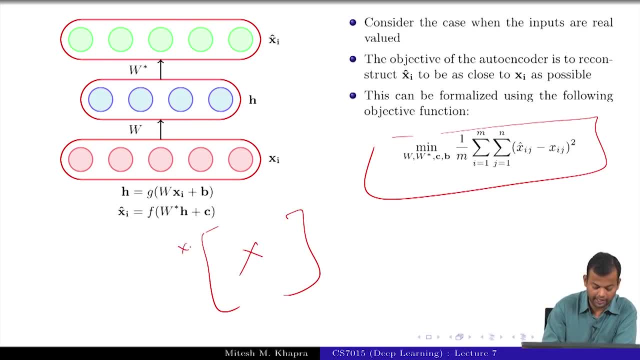 It says that for all my input data x 1 to x 2.. Right, So what does this actually capture? It says that for all my input data x 1 to x m, for each of these dimensions, x 1, 2 up to x 1 n. right, I want to make sure that my 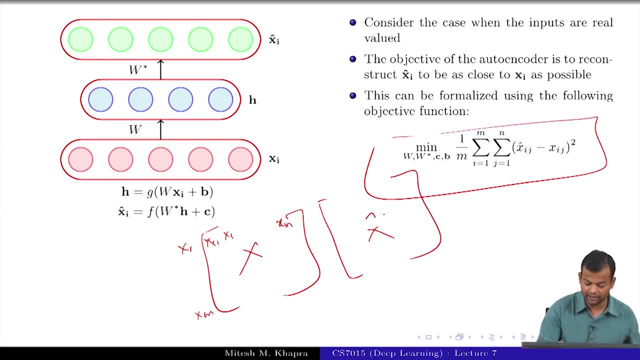 original input. I will have a similar x hat reconstructed where I will have x 1 1 hat, x 1 2 hat and x 1 n hat right. So I want to make sure that each of these pairs of variables are actually similar and I can capture that by ensuring that the squared error loss between 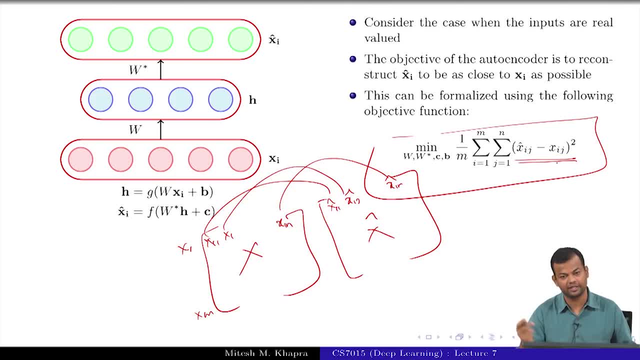 the ijth entry in my output is the same as these, or rather, I could capture the squared error loss between the ijth entry in the output and the input. ok, That is what this function is trying to capture straight forward. similar things we have seen while we were doing regression. 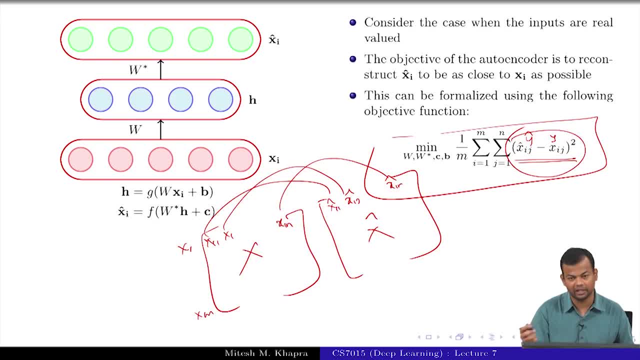 except that there we had y, hat and y, but here we are just trying to reconstruct the input, So there is no y, here we just have the x. ok, And the parameters of the objective function are of course all the variables, or all the parameters that we have in our 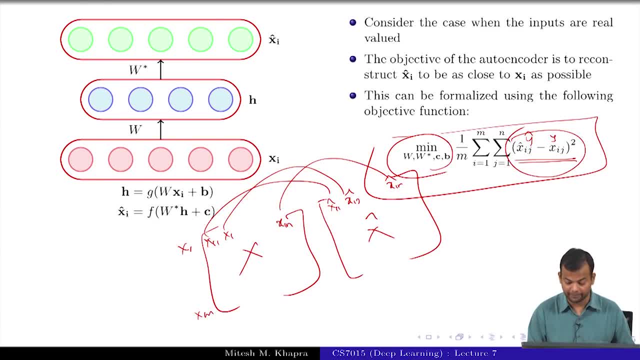 network, Whether that is W, star, c and b, ok. ok, and the matrix or the vector we are fighting? this is the following: So we have x, i. So what I am looking at here is: I have gotten rid of this summation and I am just written it in vector form. So let me just explain what 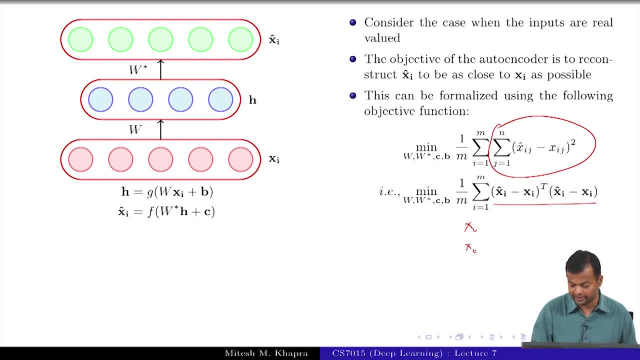 this means. So this is what x i would look like, right, So this would be: x i 1, x I 2 up to x i n. ok, this is the vector, and then you have the x i hat vector. So if I get, 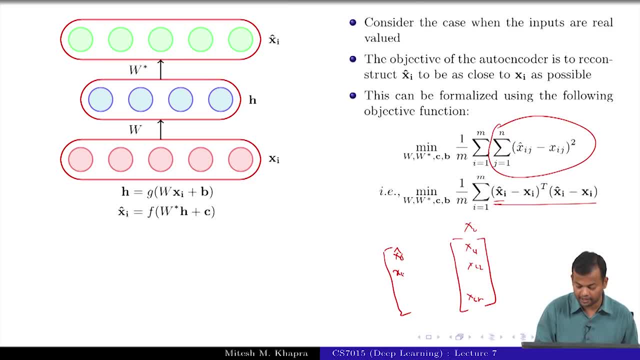 which is going to be x i 1 hat x i 2 hat up to x i n hat right. So, taking the difference between these two vectors, that is what this term is. So what you will get is essentially x i 1 hat minus x i 1 up to x i n hat minus x i n right. And then you are taking the dot. 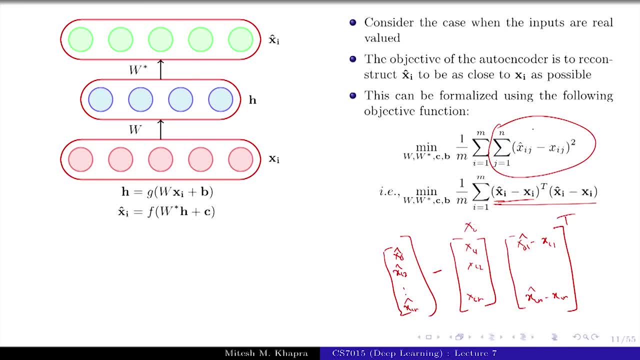 product of this vector with itself, which will essentially give you this summation, right? So the dot product of this vector with itself is actually going to be this summation. It is going to be the sum of the squares of the elements of this vector, and that is exactly. 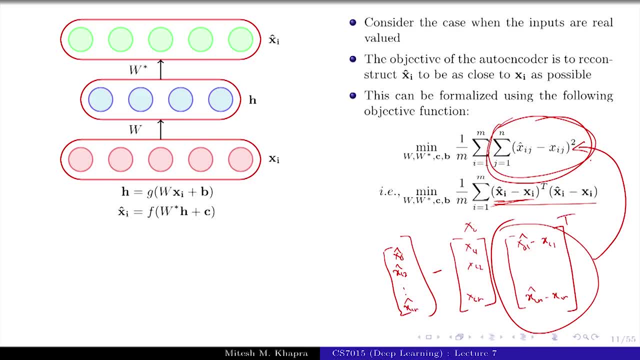 what we wanted. So this is a more compact, vectorial way of writing the same thing. ok, And now we can just train the autoencoder by treating it as a regular feed forward neural network. This is just like any other feed forward neural network. you have defined the. 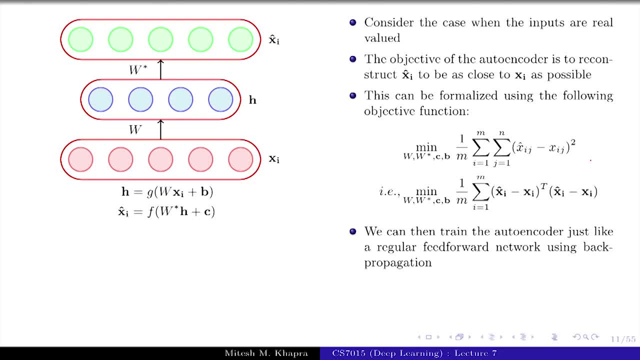 loss function and you can just use back propagation to treat it right. And in this case, all we need is a formula for the gradient of the loss function with respect to your parameters, which are w and w star. I have again ignore the biases and 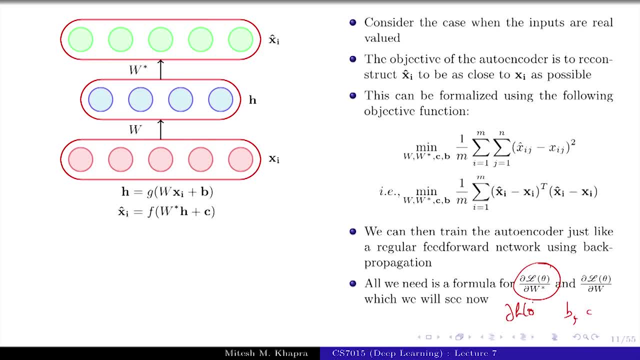 the biases here, b and c. So we will also need dou L theta by dou b and dou L theta by dou c, right? So these two gradients also you will need, but these are generally the easier ones to handle. if you know how to compute this, the b and c are very easy, ok, So let 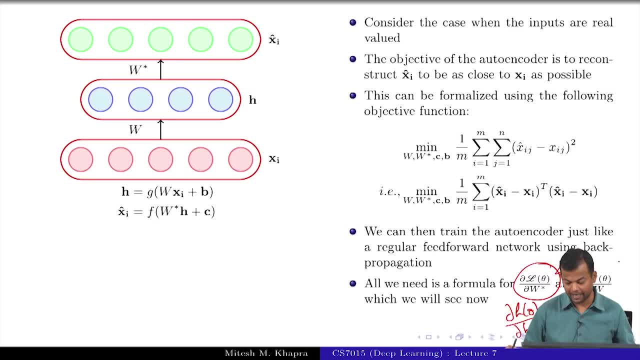 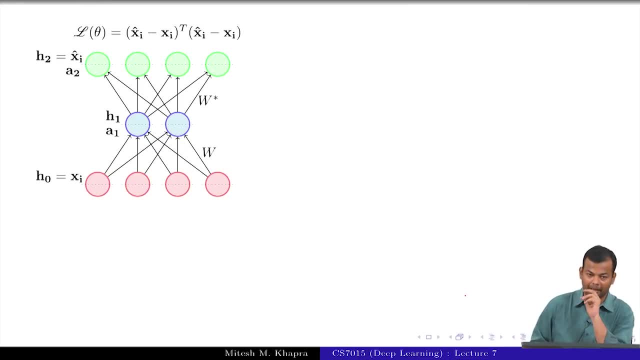 us look at this. So what we will need for back propagation, as I said, we will need this gradient, right, all these four gradients, but let us focus on one of these Now. we have already done back propagation and we have looked at arbitrary neural feed forward, neural networks here, right, 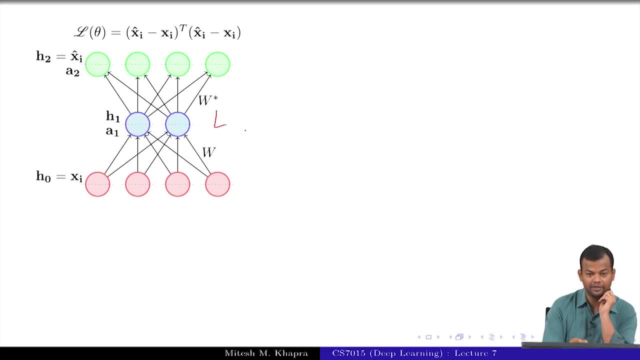 We did not have. we just said that there are L hidden layers and in this case L is equal to 1, right? or rather, we had said there was L minus 1 hidden layers and the L th layer was the output, right. So in this case L minus 1 is equal to 1. that means there is just one. 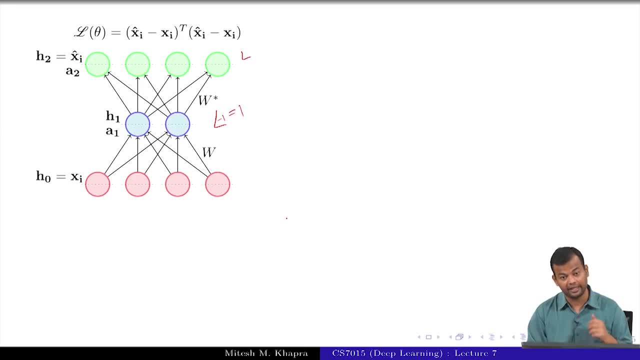 hidden layer. So it does not matter. we had actually derived it for the general case when L is equal, when the number of hidden layers is L minus 1, and here we just have one hidden layer. So it is much more simpler than what we had learned, and even for the number of. 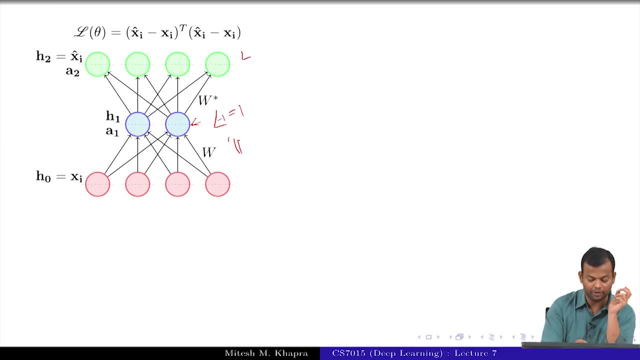 neurons in the each of these layers. we just assume, general, that it could be R, n, and in this case we would have some R d which is less than n, or it could even be greater than n, right So? but it does not matter, because, whatever. 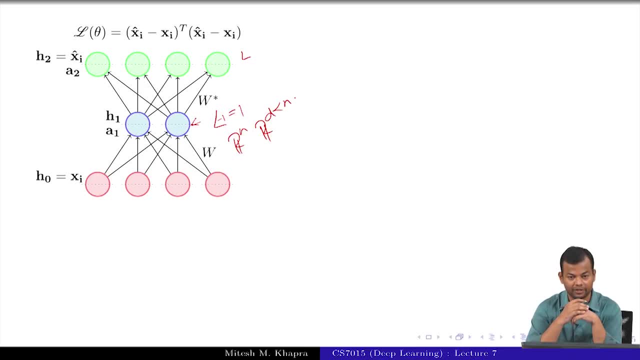 algorithm we had or whatever equations we had derived for back propagation. they did not care about what this n or d was, we just derive it in generic terms. right and the same for the output layer. right. We did not assume any number of inputs, any number of. 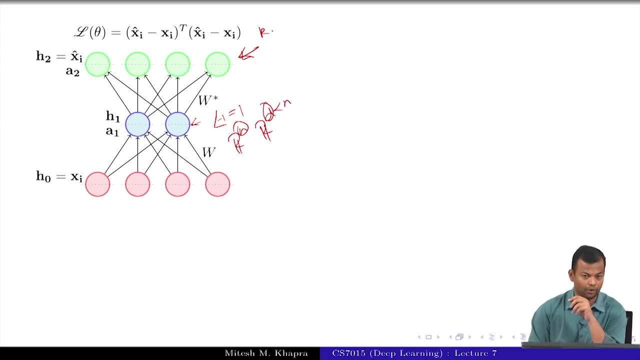 neurons in the output layer. they again said that it has some k neurons. but there the catch is. in the earlier case, when we had derived back propagation, we were dealing with classification and we had these k classes that we want to predict at the output and in which case our 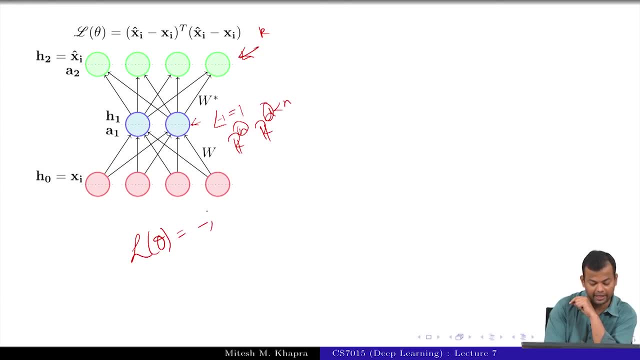 loss function was actually the cross entropy or the negative log likelihood function, right where we were trying to maximize the probability of the correct class out of the k given classes. But here our loss function is slightly different. it is actually the squared error loss between the input and the output. So now, given this difference in the loss function, does it mean? 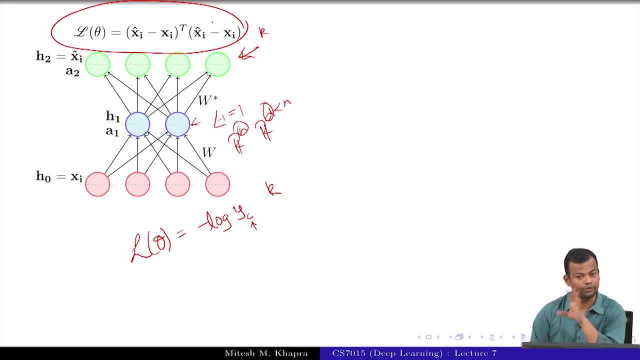 that everything that we learned in the previous lecture on back propagation. we just have to throw it all away because now there is a new loss function. That means my gradients are going to be very different from what I had derived for the back propagation loss, where I was looking at the cross entropy loss as compared to the 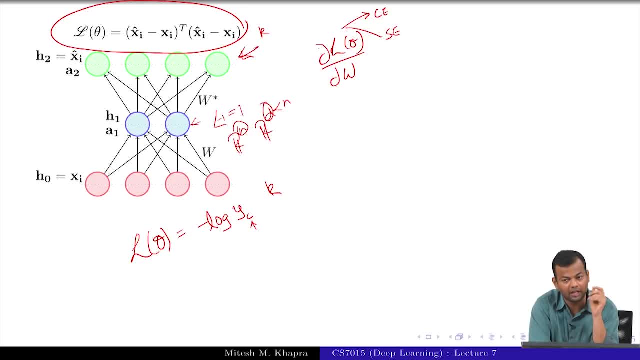 squared error loss. So does it mean that I will have to throw away all the hard work that we had done in that course, in that lecture, or can we reuse something from that we can reuse right? So let us look at what we can reuse and I will just give you an intuitive. 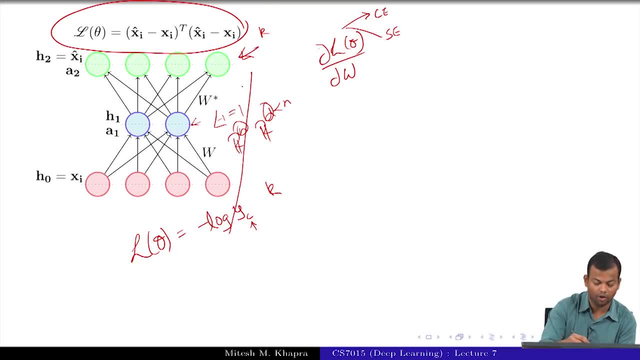 explanation for that. So you can think of this as a composite function, right? you are taking your input, passing it through a lot of functions and then arriving at the output, and then your loss function is actually a function of the output. So that is what we are going to do. So what we are going to do is that we are going to 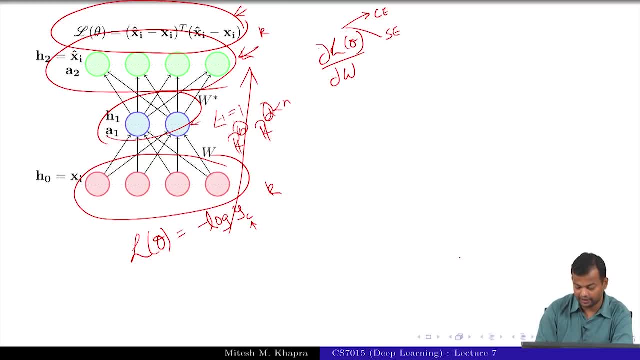 calculate. well, let us left the cela function of the output, say 0, and then called this faster. so what can we call this SW power? OK, So what we have is something like this: We have a situation like this: that you had an input x, right, you computed some function. 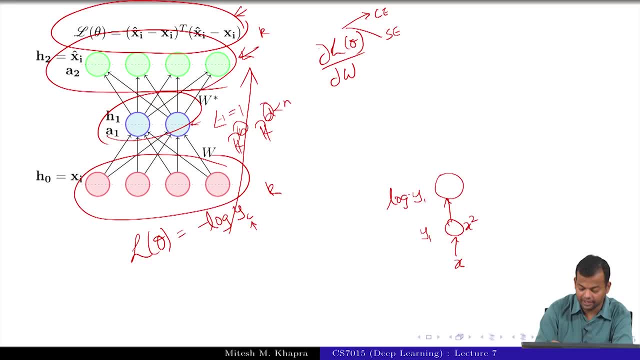 of it say x square, So I will call this as y 1. then you compute some other function of it say y 1, say log of y 1, right? So this was log of y 1.. So in effect it is actually. 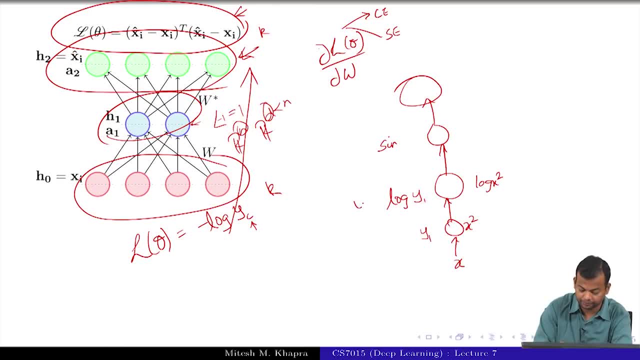 log of x square, because y 1 is equal to x square. and then some other function, and then function which was sin of- I am calling this y 2.. So say this was sin of y 2. and finally you had this function which was e raised to y 3. So you have a very complex composite. 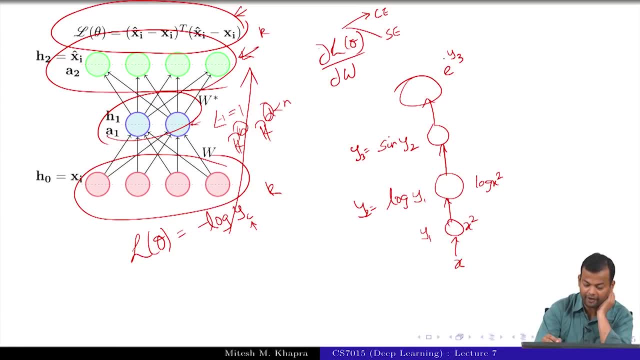 function of your original input right. and this is your final output function that you are considering, which is e raised to y 3.. Now, the way you would do this is if you want to take the gradient of d- l with respect to your input d x, right? In that case, what you 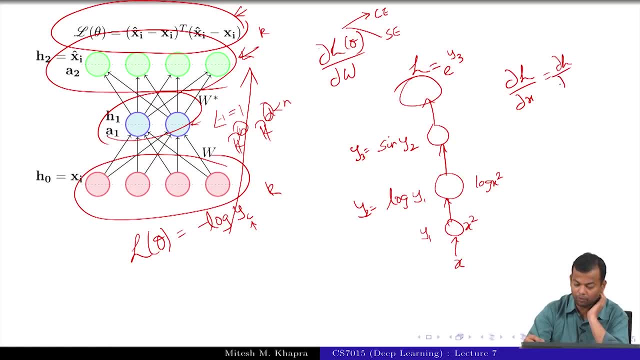 do is you just apply the chain rule. you will write it as dou l by dou y 3, dou y 3 by dou y 2, dou y 2 by dou y 1, and then dou y 1 by dou x. right, and this is something very similar. 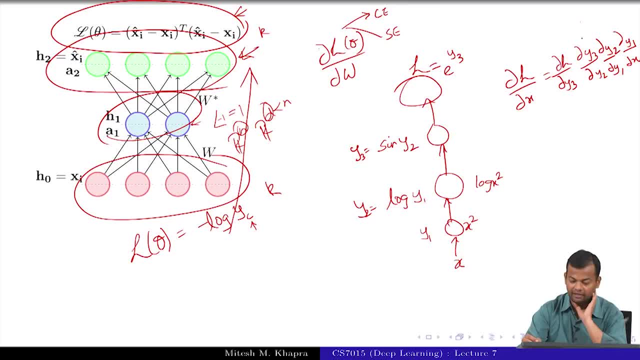 that we had done in the back propagation lecture. We had constructed this chain, and then we had attacked every element of this chain and derived how to deal with that right. So we derived a neat expression for that. Now the question which I am asking you is: 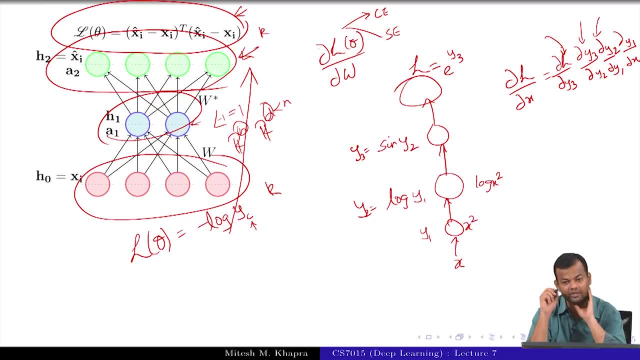 that in that lecture we had assumed a certain l and that l was actually cross entropy. but in this lecture I have actually changed the l. what I am saying is the l is actually equal to the squared error loss. Now, does that mean that I have to throw away all this work? 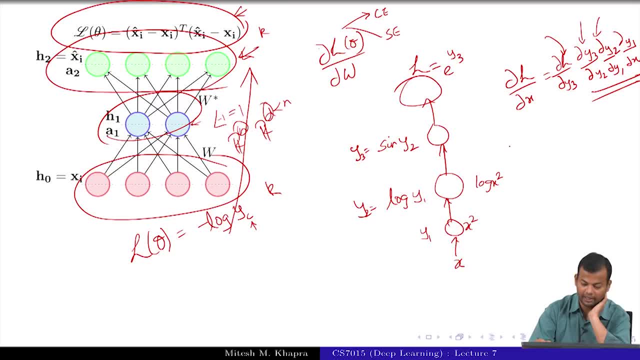 that I had done No right. So even in this example, if you look at it, suppose I change this function from e raised to y 3, to say square root of y 3, right? So I have just changed my l, right. 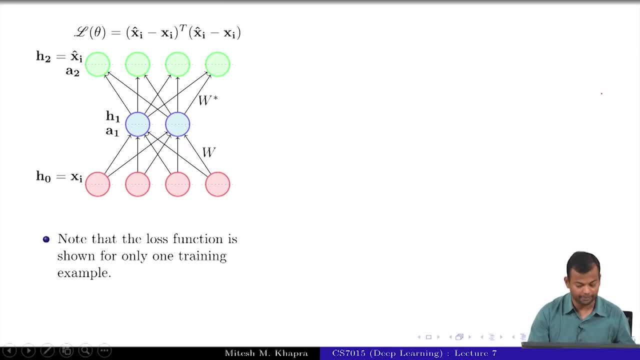 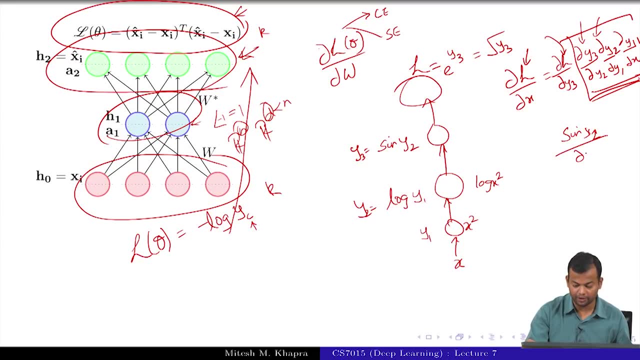 But notice that all of these other guys are going to remain the same, because y 3 is still sign of y 2. So that the derivative of y 3 with respect to y 2 is not going to change. even though I have changed the output function, the loss function, everything else is going. 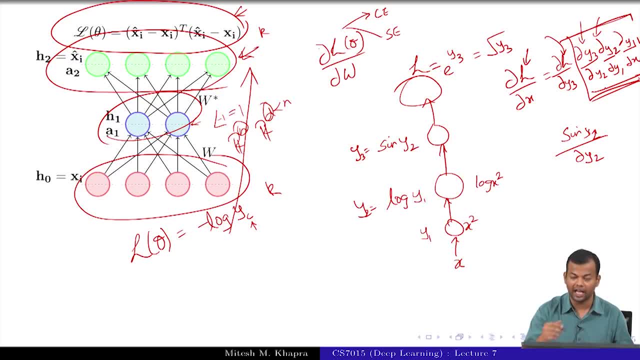 to be remaining the same right. So that means all these portions I could just reuse from the time when I had computed for this chain. I just need to rework on this final expression and plug it in right. So that is why all the work that we had done 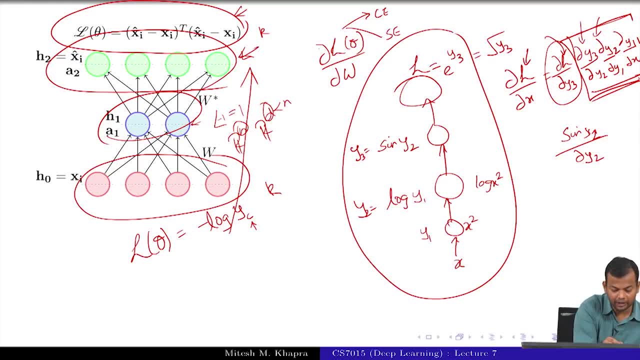 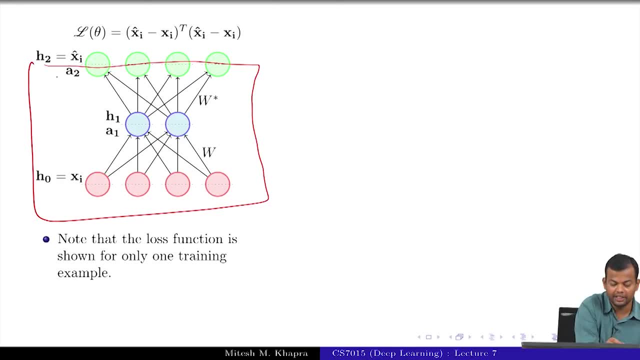 in the case of back propagation, will not go to waste, In particular everything that we had done. So let me just go to the next slide. So, in particular, everything that we had done for this portion of the network right, which is actually dou a, 2, all the way up to dou w right. So, if ok, So let me write it at: 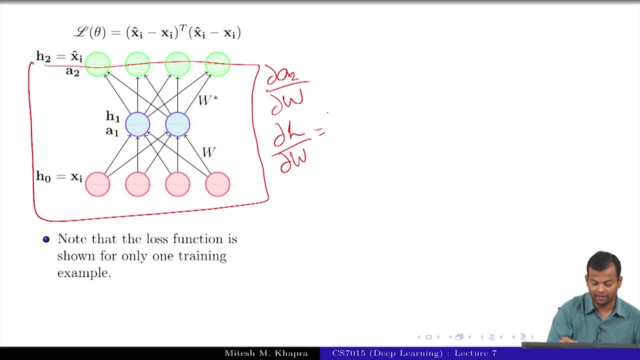 this: I want dou l by dou w, So I can write it compactly as dou l by dou a 2 and then dou a 2 by dou w, right? So this portion is not going to change, because I am not change any of the functions here. I have just assumed sigmoid or logistic or the same kind of network. 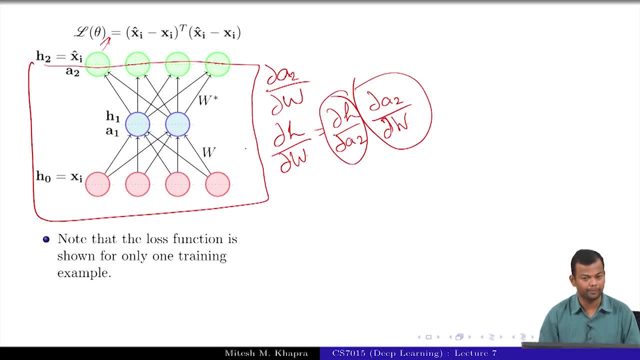 The only thing I have changed is something at the output layer, So I will just need to re compute this and the rest of it can be reused, right? So that is the intuition which I wanted to give you, and that is exactly what is written on this slide. So I am written. 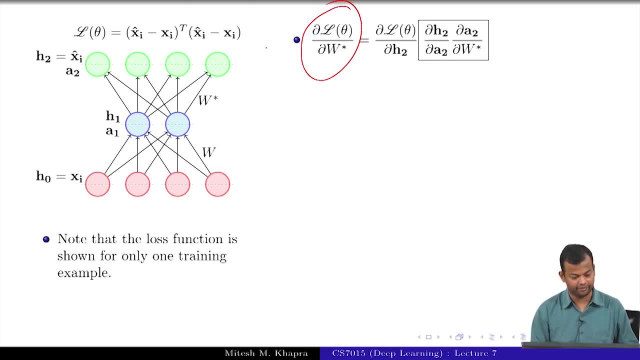 it as dou l theta by dou w star. that is the first gradient I have interested in and I could write it. So I can write it as dou l theta by dou w star and I could write it as dou l theta by dou h 2, dou h 2 by a 2 and dou a 2 by w star. right Now, this portion. 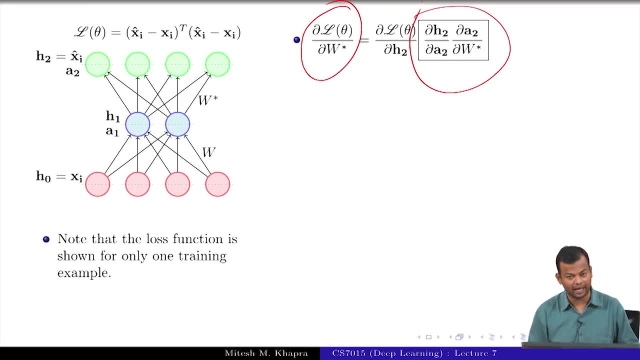 as I was trying to say, is something that we have already seen in the back propagation lecture, and nothing has changed in the network in that part, So you can just reuse it as it is, and this portion is something that we need to re compute right. that is the only. 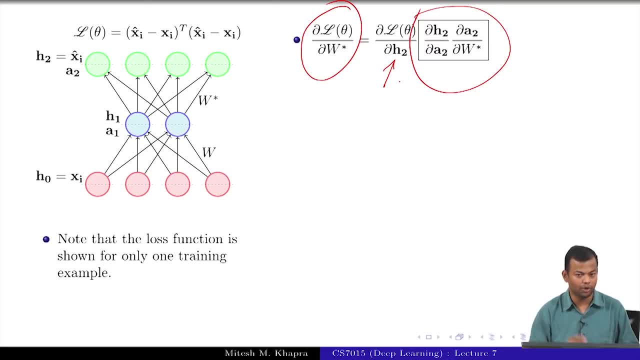 thing that we need to re compute and plug it into our back propagation code or the algorithm which we had in the previous lecture, And similarly, if you want to do dou l theta by dou w, So it is the same idea here- that you could write it as the following chain: and this part: 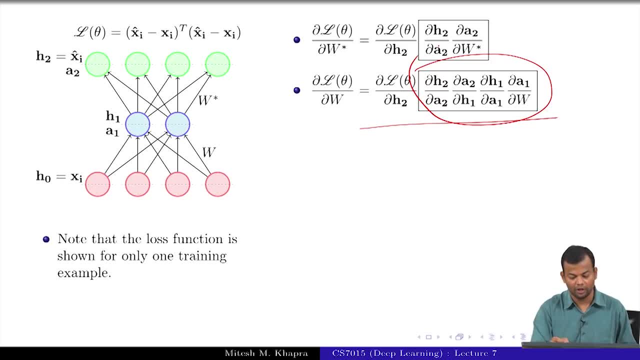 of the chain. you already know how to compute from the back propagation lecture. All you need to do is change the loss function and just try to find the derivative of the loss function with respect to your output layer, which is h 2. that is the final thing that 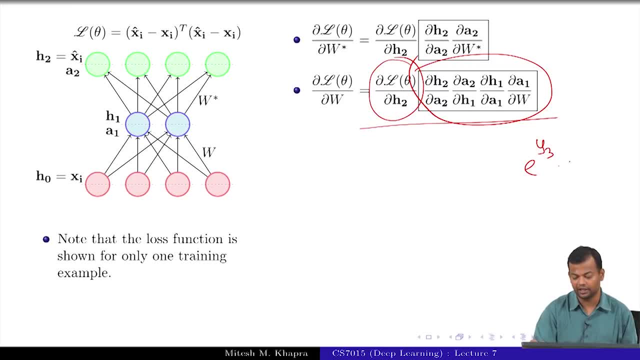 you have changed, just as in my toy example, I had changed e raise to y 3, to square root of y 3, right? that is the similar change that I am trying to do here. fine, So all we need to do is dou l theta by dou h 2, but dou h 2 is the same as x. i hat right, because that. 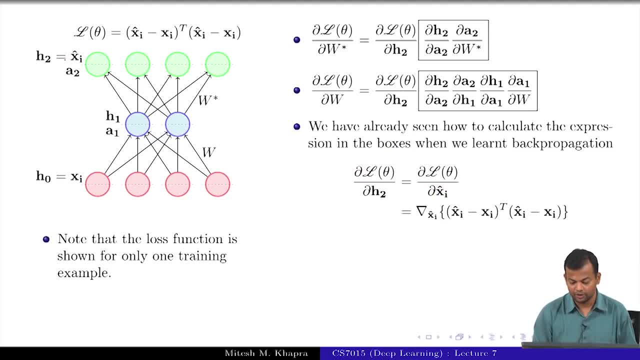 is my output and my output I am calling it as x i hat. So I need to take actually the derivative of this, So I am just using the vector form here. I could have also written it as this: summation over: i equal to 1 to n x. i j minus x hat i j the whole square right. 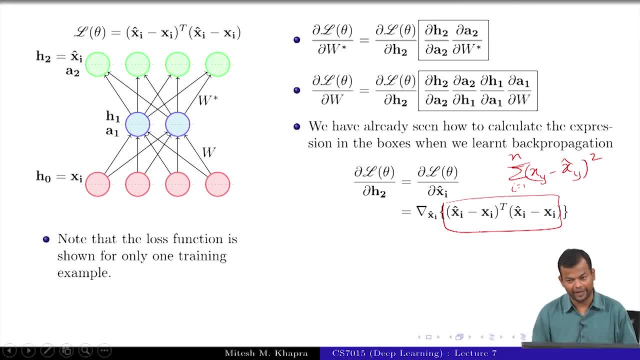 I could have also written it. I am just writing it as a vector here, in the vector form here, right, but this quantity, ultimately, is going to be a scalar because it is a dot product between two vectors, which is a scalar. So what I am doing here is taking the derivative. 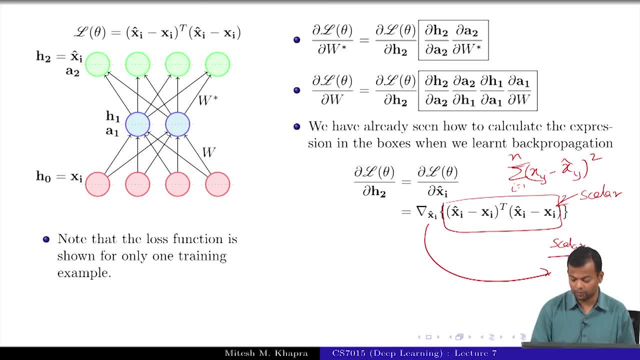 of a scalar with respect to this vector. So what is that derivative going to be? it is going to be a vector, ok, and I am just So. we have done similar stuff in the past, So you can actually easily work this out. So this will actually turn out to be the following: 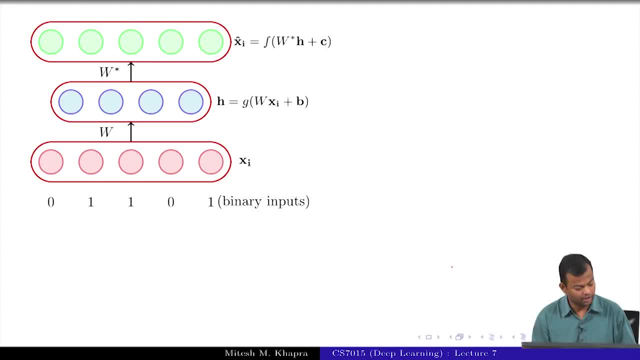 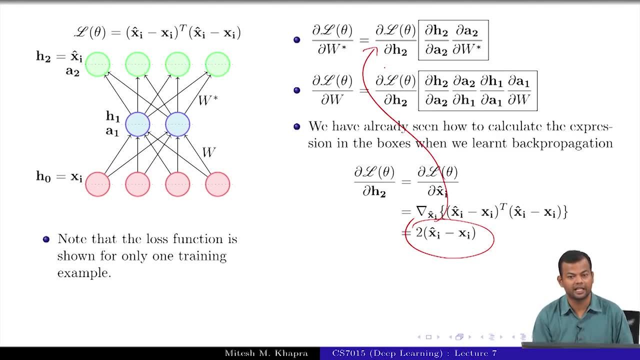 vector which is 2 times x. i hat minus x, i right. So this is very simple. I have just computed this and all I need to do is go back and change my back propagation code and change this derivative of the loss function with respect to the output. 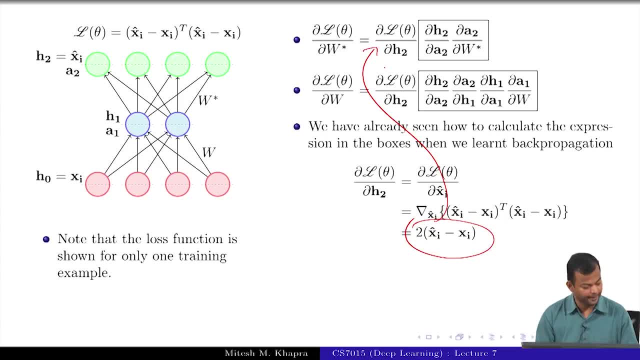 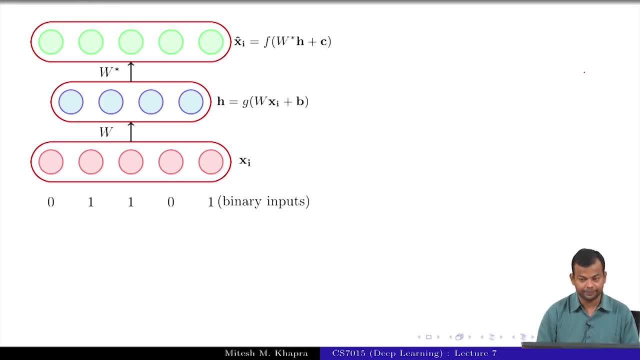 layer and the rest of the code. I can just reuse it as it is. ok. So now, similarly. So we have both of these ready, ok. Now let us look at the other case, when we have binary inputs. ok, This is the most more. this is something different that we will have to do here. So 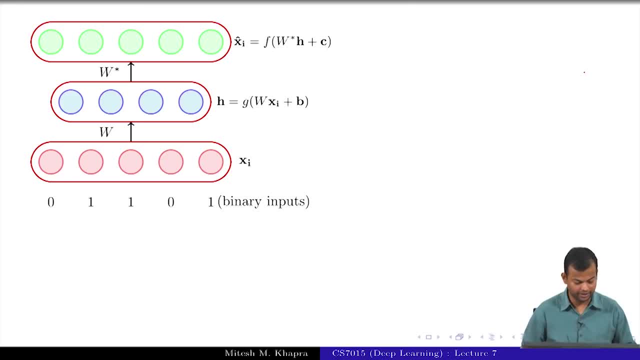 we will now look at the second case, where the inputs are binary. ok, So we have the first. we look at the case when the inputs were real numbers and hence your outputs also needed to be real numbers. Now we look at the case where the inputs are. 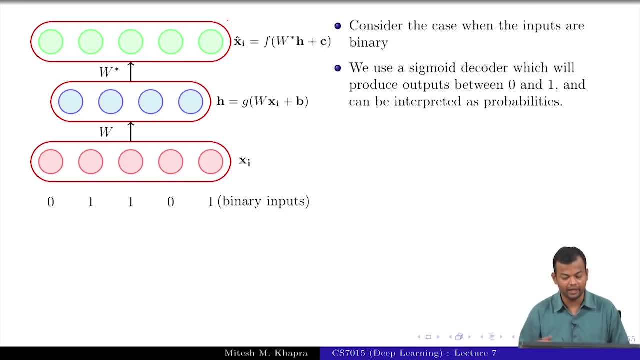 binary, and hence your outputs also need to be binary. ok, Now here. so each of these guys is actually a sigmoid function, say it is an, or rather, if you look at the output, you could divide into two parts. So this is the pre activation and this is the activation right. 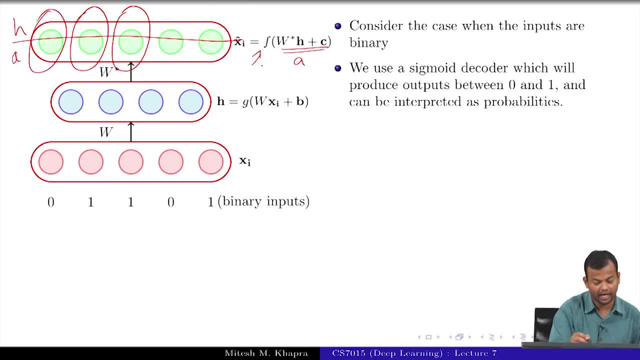 So, Yeah, Yeah, function and this is the activation, right? So this activation is actually chosen as a sigmoid function or the actually the logistic function, not the sigmoid function. of course, logistic is a sigmoid function, but the logistic function, which was 1 over 1 plus e, raise to. 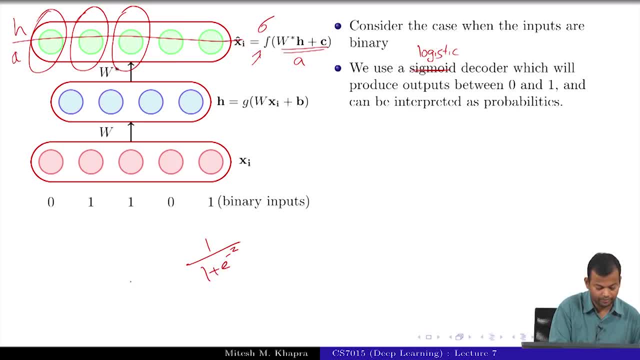 minus z, right, So logistic of z is equal to 1 over 1 plus e. raise to minus z. ok, Remember that the sigmoid function was element wise. that means this: a is a vector, it has elements a 1, a 2, up to a n, and then, you know, apply the sigmoid to it, you get h, which is: 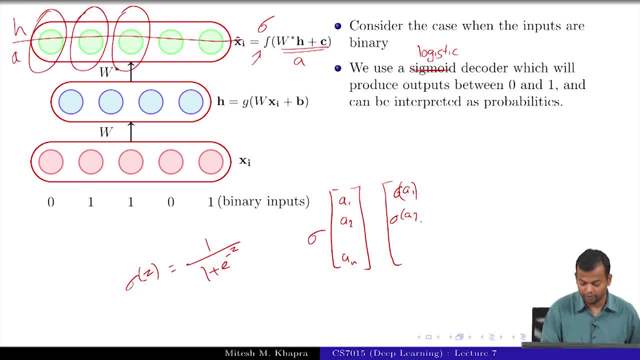 going to be sigmoid of a 1, sigmoid of a 2 and sigmoid of a n, right? So it is just the sigmoid applied to every element of the activation layer, that means every element of this vector which I have circled. ok. 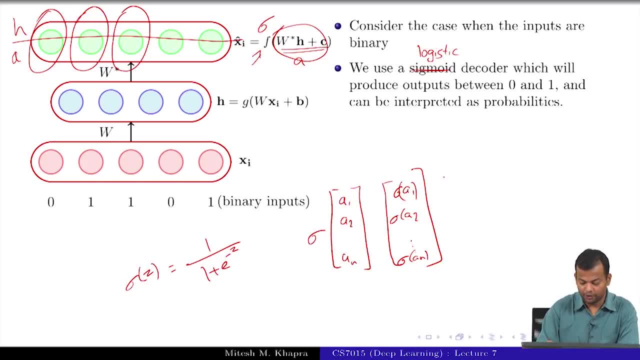 So now, in this case, So your outputs are going to be between 0 to 1, right, because your inputs were also between 0 to 1 and your sigmoid, or the logistic function, is going to give you clamped outputs between 0 to 1.. So, since this is between 0 to 1, we could actually interpret it as: 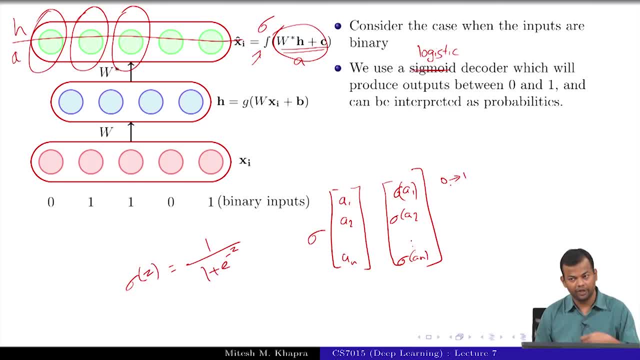 probabilities right. So we could say that whatever you are reconstructing is actually telling you that with 0.8, suppose the reconstruction value is 0.8, then you could think of it that with probability 0.8, it is telling you that the output should have been 1, right? and if 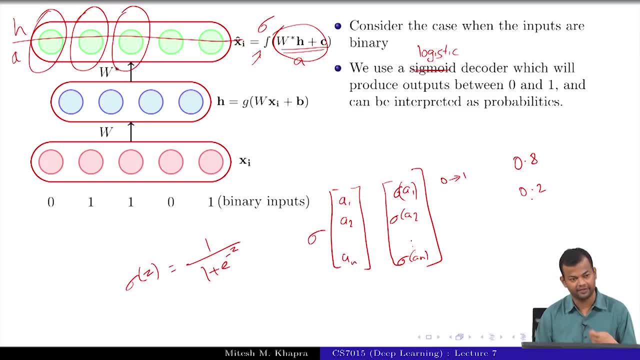 it tells you that the output should have been 1, right. and if it tells you that the output is 0.2, if the sigmoid gives an output as 0.2, then you could think of it that with probability 0.2, the output was actually 0, or rather the input was 0, because your input 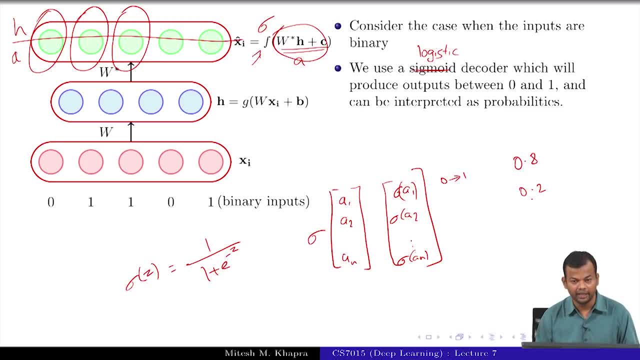 is the same as the output, right? So that is one way of interpreting it and this way of interpreting it. why does it make sense? So we will just look at that, right. So before that, if we I do not give you this interpretation, and remember that the sigmoid 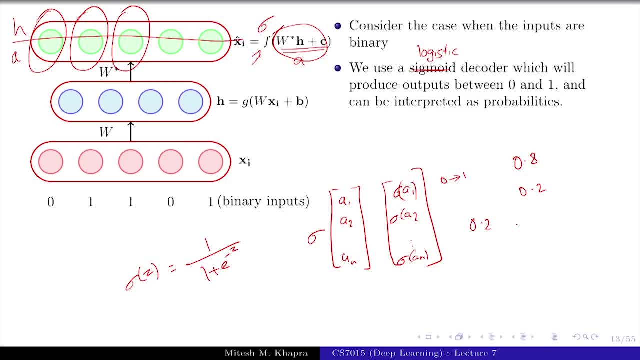 is going to produce values between 0 to 1,, but not necessarily 0 and 1,. right, It will try to be as close to 0 and the input is 0,, but it could also produce 0.0, 5 and so on. 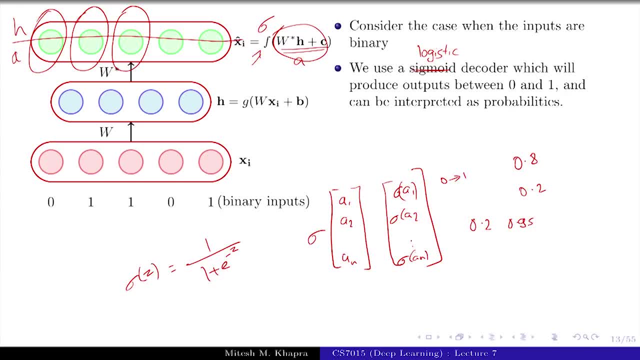 and when the output is 0.9, it could also produce something like 0.95.. So at the output also, you are going to get these vectors, which are of which will look something like this, right, and suppose your input was 0, 1,, 0, 1.. Now can you think of a suitable loss function? 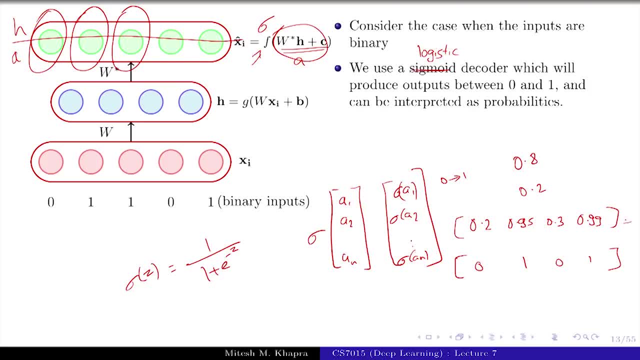 for this. So, again, these are two vectors. these are x, hat and x. So, once again, you, you could have just gone with the with the squared error loss, right? you could have taken the squared error difference between these two and you could have been fine, right. 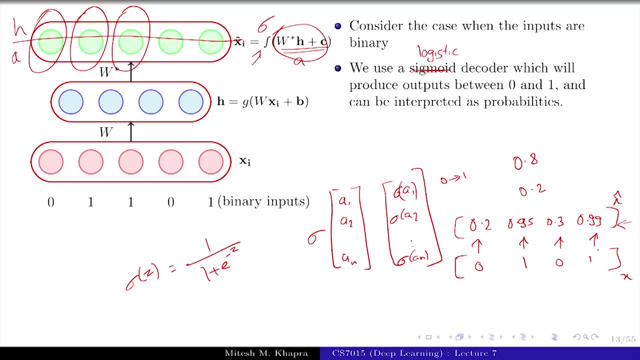 So that is definitely one way of going about it, but whenever we are looking at these binary inputs and whenever this probabilistic interpretation is possible, we tend to do something better, which is look at the cross entropy loss instead of looking at the squared error loss. 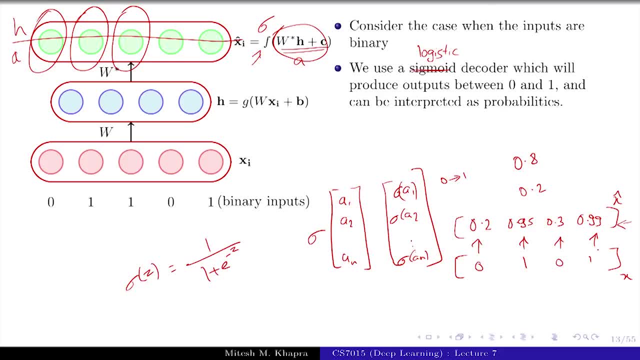 So I am not saying that the squared error loss is wrong in this case, but you could also use this cross entropy loss and, in practice, for our binary inputs, the cross entropy loss often works much better than the squared error loss, right? So let us see what I mean by the cross entropy loss. 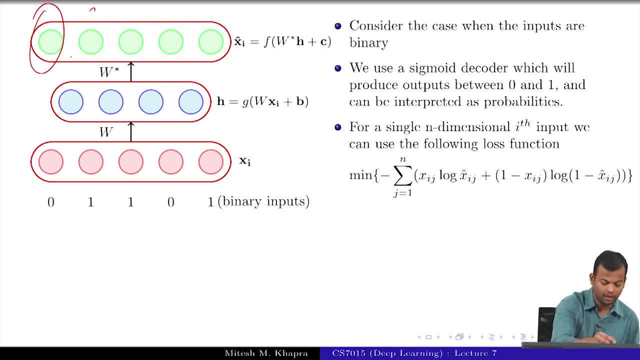 So remember that you have n outputs, right? that is why this summation: let us not worry too much about what is written inside for the time being. I will explain that, but that is the. I just want to explain the summation first. So what you are saying is that for each of these green guys at the output, you are going 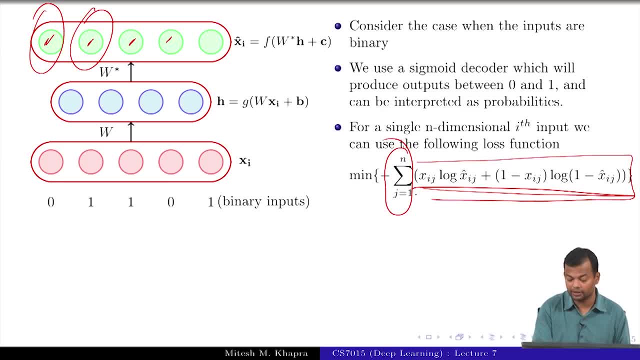 to make some, Some loss and you just want to sum over that loss. that is what we are trying to see Now. ideally, you could have just written it as just done what you had done before, and written this entire, replace this entire box by this squared error loss, and that would. 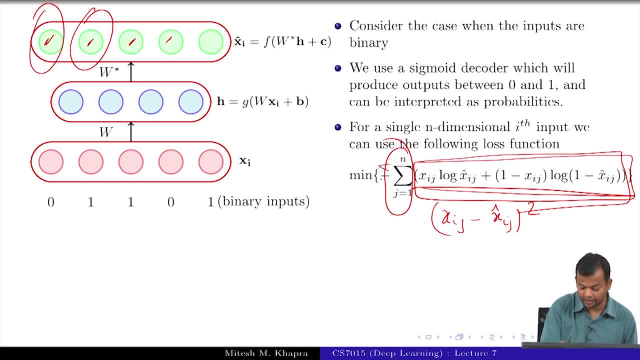 have been just fine, right. Of course there should have also have been this summation: i equal to 1 to m here, because you are going over all the m training instances and for each of the m training instances you are trying to minimize this loss. 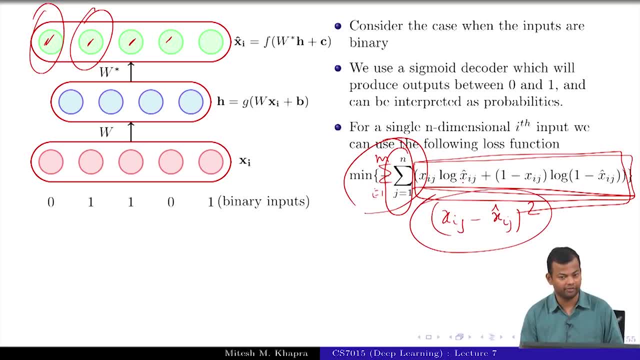 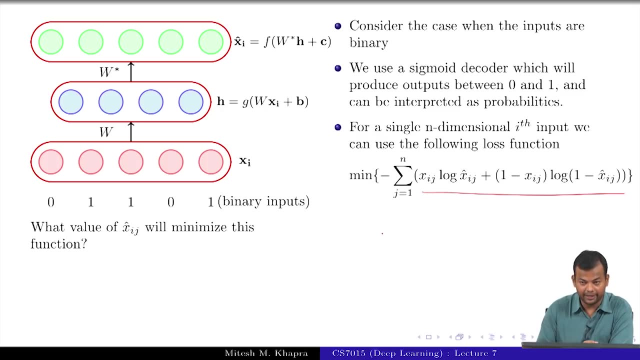 So this two summations, Just followed by the squared error loss, would just have been fine, but instead of that, I have this something special here. ok, So let us look at what this special quantity is. ok, And now for that. remember that I am trying to interpret each of these inputs as a binary. 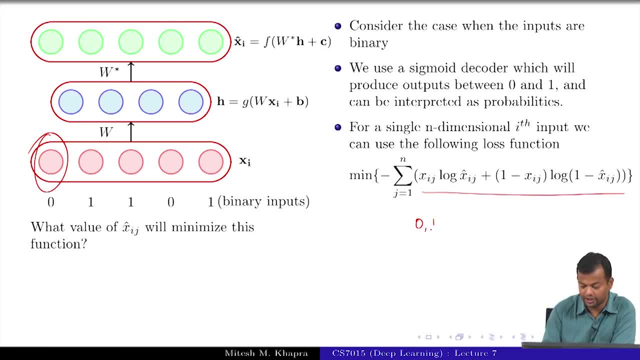 random variable. I am saying that they can take values 0 or 1.. So I can think of it that when I am given that this value is 0. I can write it as this: So this is a deterministic probability distribution where I have p and the probability mass is: 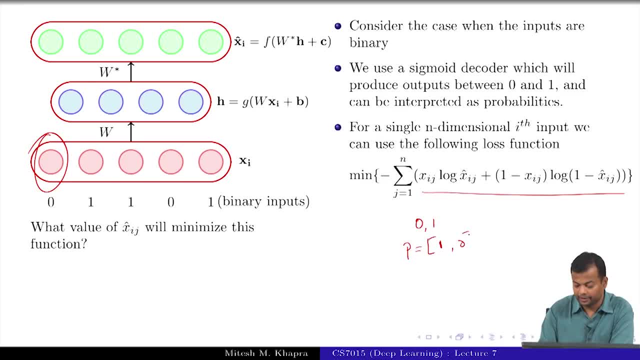 entirely concentrated on the 0 value and my the probability mass on the value 1 is 0.. This is something similar to what we had done earlier when we were given these labels- suppose it was apple, orange, mango and banana- and the class label was given to us that this is an. 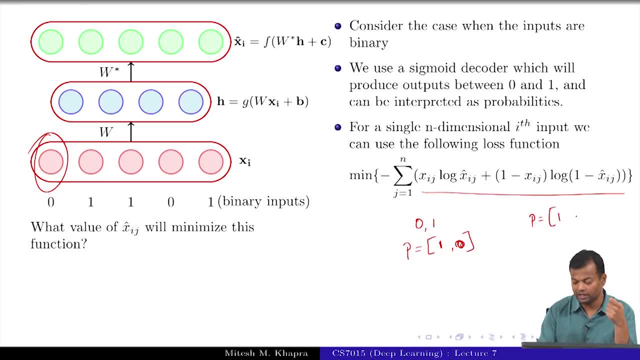 apple, then we could still write it as a probability distribution where all the mass was concentrated on apple and everything else was 0. So I am saying something similar here, right? So you could think of it, So that two possible values can occur here, 1 and 0. and if I tell you this is 0, right? 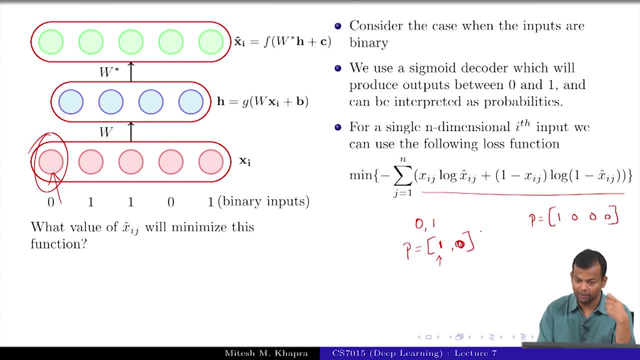 then I am telling you that with probability 1 it is 0 and with probability 0 it is 0. So I can still write it as a probability distribution, Now the same thing I can have at the output. So for this unit, when I am trying to reconstruct it, and if I produce the output as 0.2, then 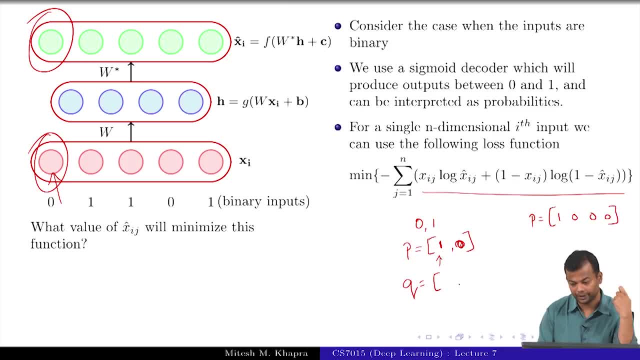 I can, or rather, let us say 0.8, then I can say that with 0.8 probability I am predicting 0.. Ok, So now I can think of this again as two probability distributions, and once I have two probability distributions I know that cross entropy is the right or a better loss function to look. 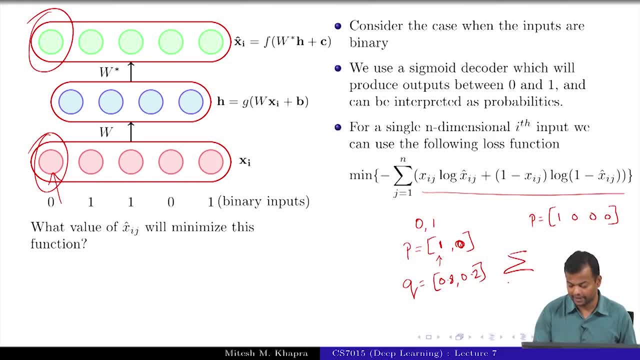 at right. And what is cross entropy? actually, in this case it would be given by summation: i equal to 1 to 2, right, or rather i equal to 0 to 1, because it those are the two values. it can take p of i right into log of q i. 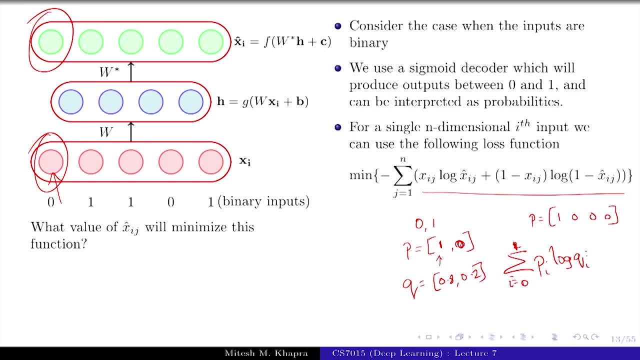 Right, Ok, Ok, So p of i into log of q i. plus, yeah, so p of i into log of q i. that is how I can write it. Ok, So let me just, since there are only two terms, I can just expand this summation, right. 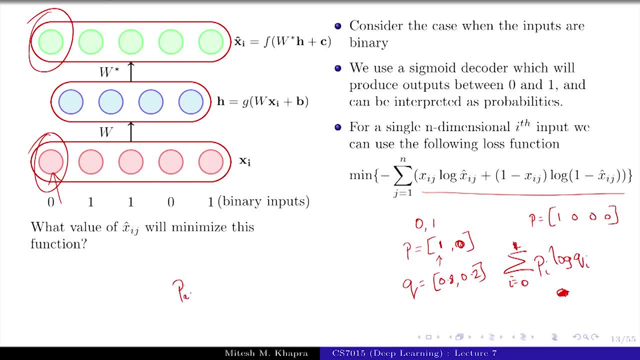 So I can write it as p i, or rather p 0. log of q 0 plus. of course there is a minus sign here. there is a minus sign at the out p 1. log of q 1.. I can just open up. 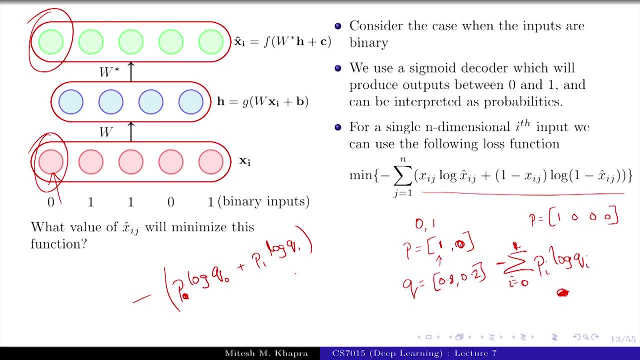 Right, Because there are only two terms, So I can write it as this. is that fine, ok. Now also, I know that there is this relation between p 0 and p 1. right, that p 0 is actually 1 minus p 1.. 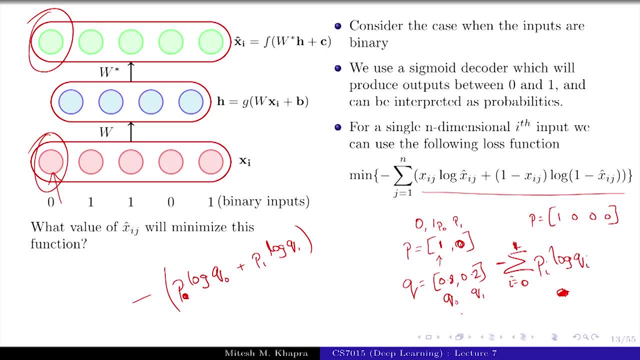 Similarly have this relation between q 0 and q 1, that q 1 is equal to 1 minus q 0, because the sum is going to be 1.. Ok, Now let us look at this sum Right case. this sum becomes interesting because now suppose your input x, i, j, right, which is: 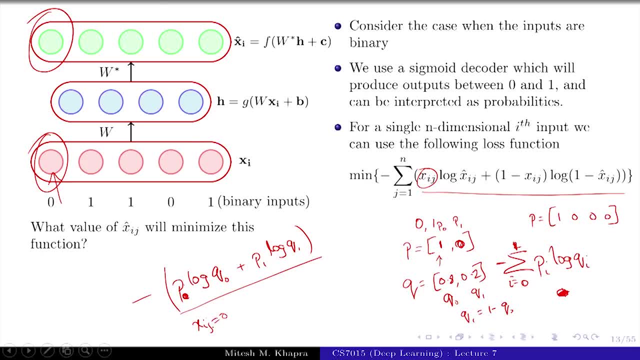 the entry that I am looking at. suppose that was equal to 0. In which case all the probability mass would be concentrated on p 0 and p 1 would actually be equal to 0, which means the second term would disappear. ok, On the other hand, if x, i, j is equal to 1, then the reverse. 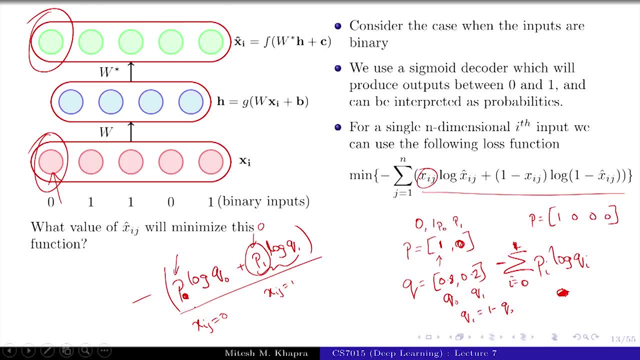 situation would happen that everything would be concentrated on p 1. that means p 1 is equal to 1, and this chi would become 0, because p 0 is going to be 0, right, ok? So there is this another way of writing it that you could say: that instead of x, instead. 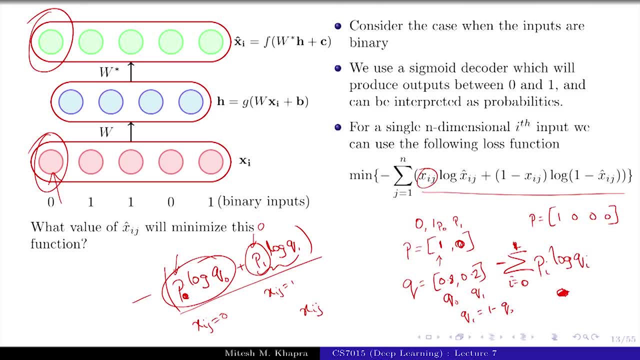 of writing p 0 and p 1, you could just write it as x i j right into log q 0 plus 1 minus x i j into log of q 1.. So now let us look at it again. So when x i j is 0, first which? 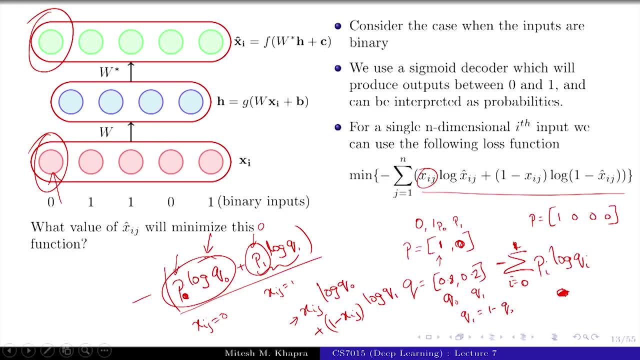 is the 0. 0.. So this is the same which happened here. the same thing, right, because whenever x, i, j is 0, p 0 is equal to sorry. sorry, it should have been q 1 and log q 0. sorry, I made a mistake. 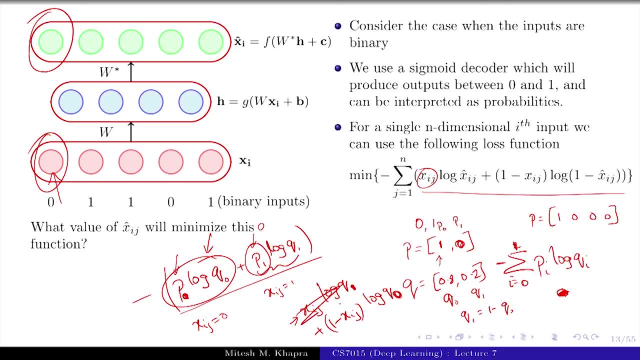 here. So it should have been: x i j into log q 1.. So, or rather, let me just rewrite it. So this is going to be. actually I can write it thus, as I look at this term first, So I can write it as x i j into log q 1, and then the second term, I am going to write it as: 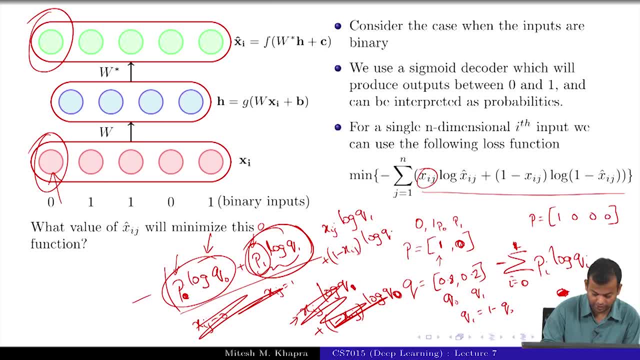 1 minus x i j into log of q 0, right, and then I am going to simplify this further, but let us see what is the consequence of this. So now, whenever x i j is equal to 1, this term will remain and the second term will disappear, and that is exactly what was happening in. 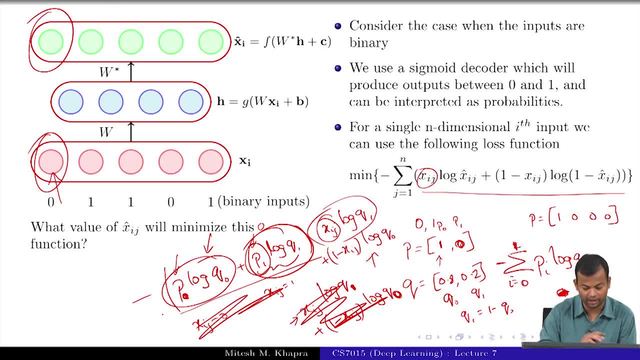 our original formula right. So this is just an equivalent way of writing. But x i, j is equal to 0. this term will disappear, but this term will remain. that means log q 0 will remain is exactly what was happening in our original formula right. So that is So now. 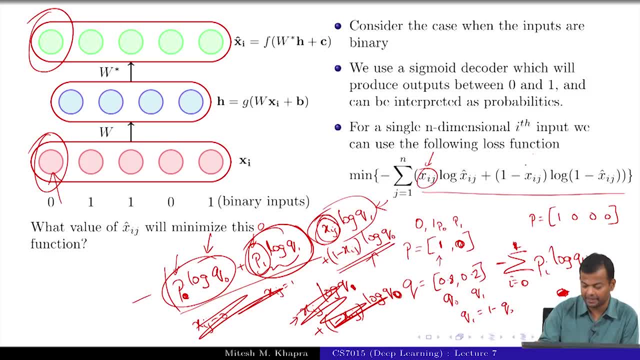 I have given you why. I can replace p 0 and p 1, or rather p 1 and p 0, by x i j and 1 minus x i j, and now I can make a similar argument for x hat i j also. So I can think of q 0. 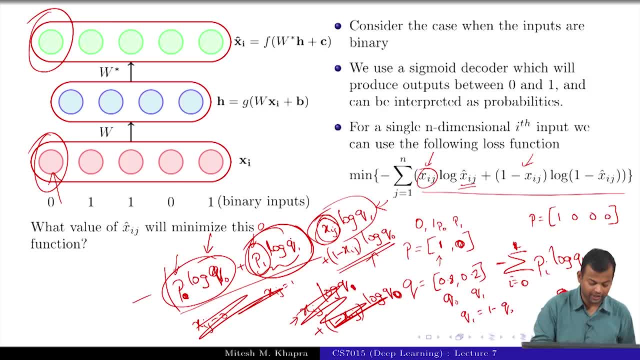 as whatever is predicted at the output, right. So sorry, I can treat q 1 as whatever is predicted about 1 output. So whatever my sigmoid function predicts, I can think of it as it is predicting the probability of getting a 1 right. So it is just predicting the heads probability. 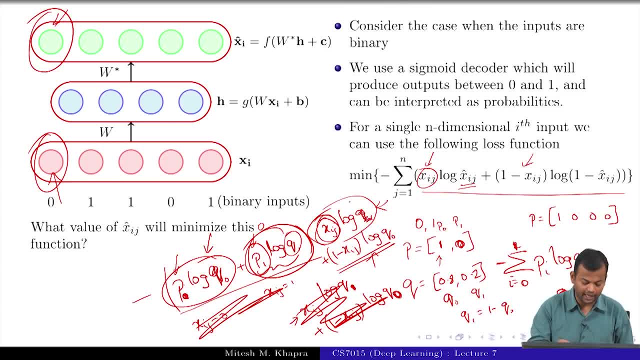 or the probability of getting 1.. So I can, instead of q i, q 1, I can write it as x i j hat, and similarly, instead of q 0, I can write it as 1 minus x i hat i j right. So did you. 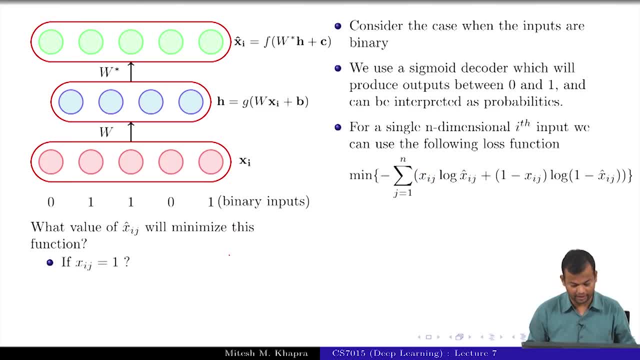 get that, So this become very messy. So let me just clean this up and I will just go over this again, right? So what I was trying to tell you is that, in the ideal case, you could have just replaced this by the squared error loss, but since you are dealing with binary inputs, 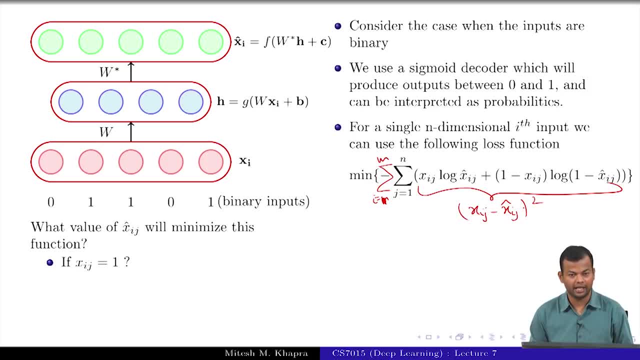 you can do something better, Because you can interpret the outputs as probabilities. So when you get a point 2 here, you can interpret it as it is telling you that the probability of this unit, China, 0.2. it is very less, and that is the same as saying that the probability of this unit being 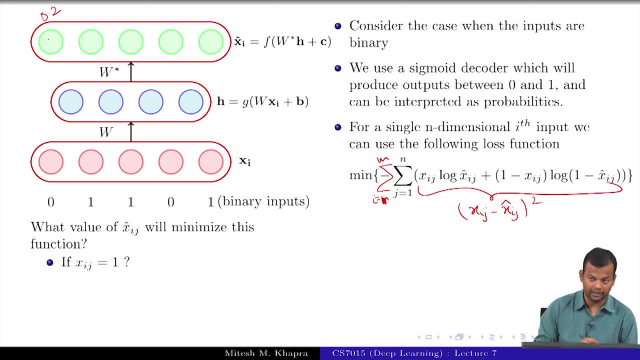 0 is 1, right, So you can interpret this as a probability. Now, if you think of it that way, then you can say that at the input you are actually given a probability distribution, So which tells you that, in the first case, your probability. 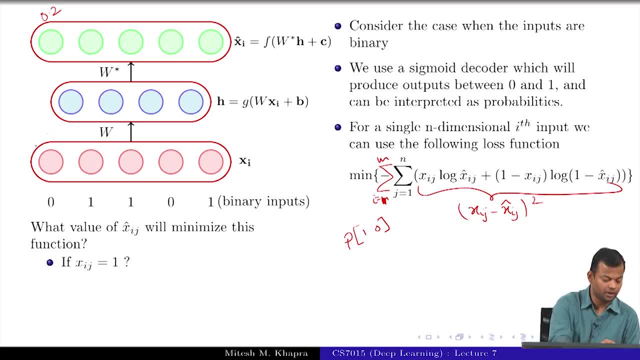 distribution looks like 1: 0, right, because all the mass is focused on the value 0, because your input is 0 at that case. And now suppose your output was 0.2. right, and 0.2 is what you are treating as a probability of. So this is the probability of 1. this is the probability. 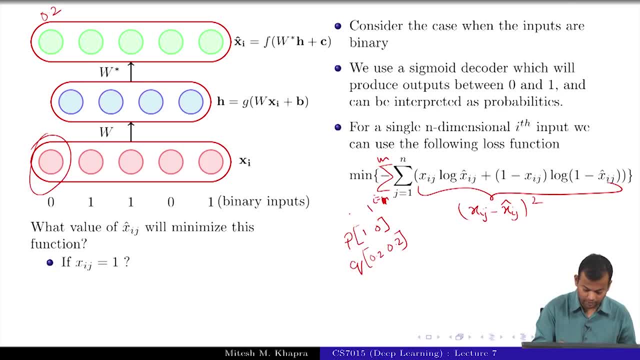 of. sorry, this is the probability of 0. oops, and this is the probability of 1. ok, So if your output is predicting 0.2, that means it is predicting 0.8 for 0 and 0.2 for 1, ok, 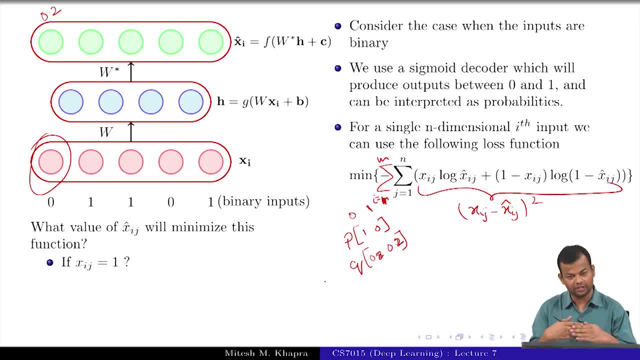 Now, if you think of it this way, then you can capture the loss function between these two guys using the cross entropy formula, which is going to be summation: i equal to 0 to 1, p, i log q. i. is that fine, ok? And now I just said that the, since there are only 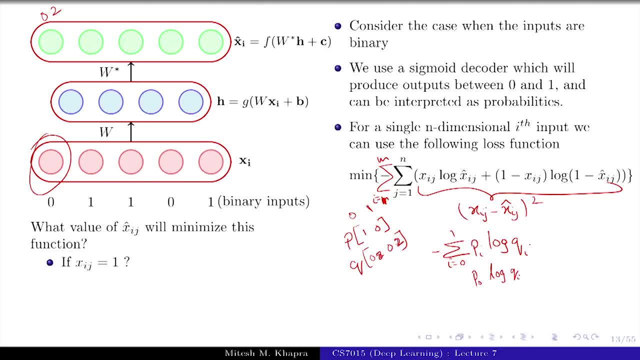 two terms. I can just write it as p 0- log q 0 plus p 1- log- q 1.. Then I focused on this relation between p 0, p 1 and your input. So whenever your input is 0, your p 0 is going. 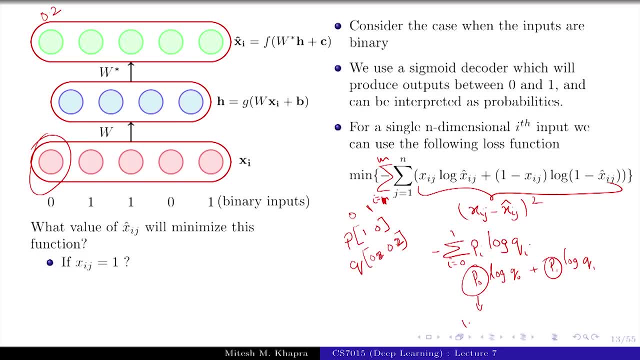 to be 1.. So then I can just replace p 0 by 1 minus my input. ok, So if the input is 0, then this guy is going to be 1, and that is exactly what this expression is also going to be. So I can write it as 1 minus x, j, log, q, 0 and similarly for the second guy whenever. 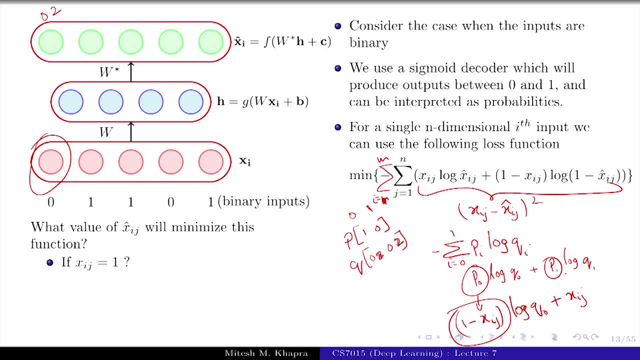 my input is 1.. This guy is going to be 1 whenever my input is. whenever my input is 1, this p 1 is going to be 1. whenever my input is 0, this p 1 is going to be 0. So I can just replace p 1. 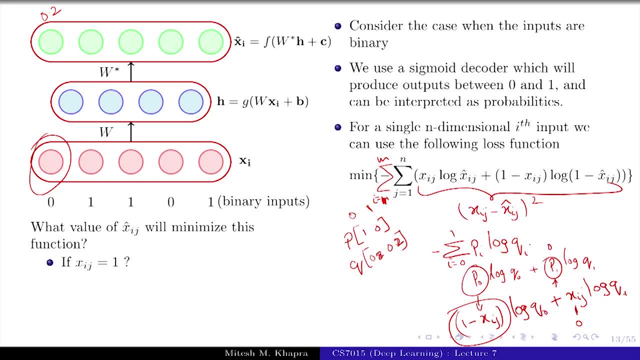 by log, by x i, j, and now you can see that this expression evaluates to the same as this expression. ok, You can substitute the value of x i j, 0 or 1. you will get the corresponding p 0, p 1, which would be 1 or 0, depending on what your input. 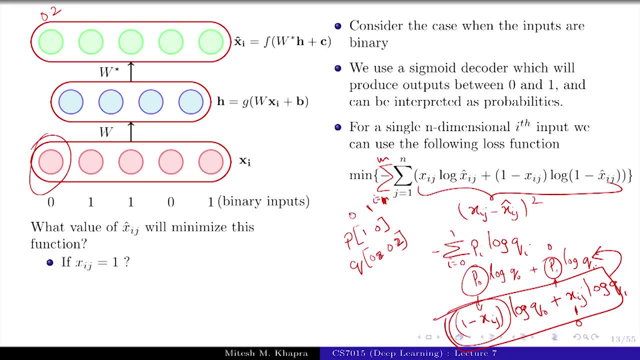 was, and these 2 expressions will evaluate to the same thing. So, just as I replace the p's by x i's, x i, j, s, I can similarly replaced by the q's by x i j. hatch right, Because once again, q 0 is nothing but 1 minus. whatever my output was predicted, because whatever 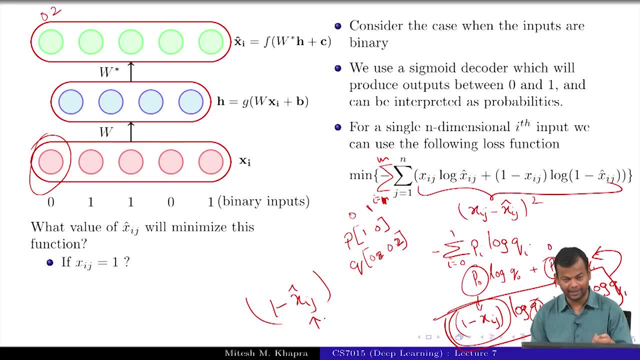 is predicted, I am treating it as the probability of the getting a 1.. So 1 minus that is going to be the probability of getting a 0. So that is what q 0 is, and similarly q 1. I can x, hat, i j, and so that is exactly what I have done in this expression here. So now this: 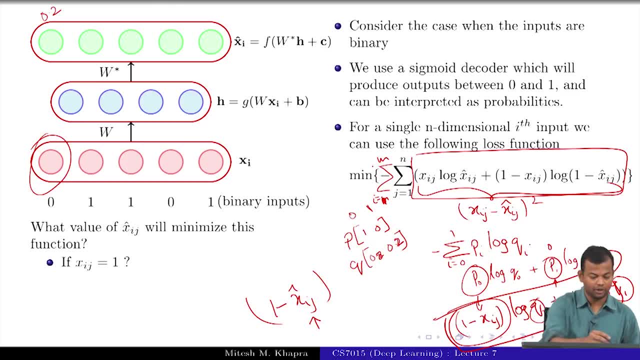 expression every term in these n terms captures the cross entropy for that particular random variable, right. So this is the original distribution p for this random variable. this is the predicted distribution q for this random variable and I have just told you that this the cross entropy. 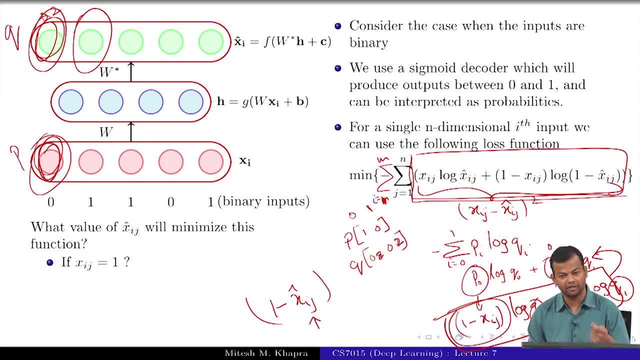 between these two distributions can be written in this simple form as a function of x i j and x hat i j. So this is a standard thing to do when you are dealing with Bernoulli random variables. So you can go back and read up a bit about it, but for now I guess 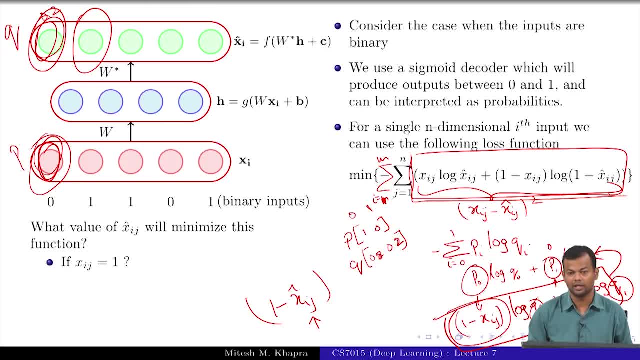 with this explanation, it should suffice to know why this expression is used and remember that. I am not telling you that the squared error function was bad. I am just telling you that, instead of the squared error function, cross entropy loss function works better when you are dealing with binary inputs. ok, fine. 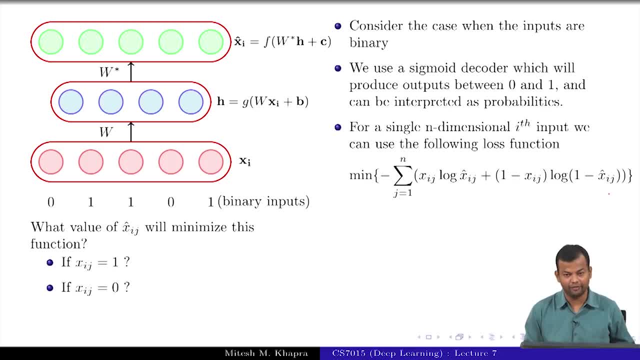 So with that, Let us pursue it. and the another way of looking at it is the following: you can now look at this expression and tell me, when is this expression going to be minimized? ok, So we have x i j and x hat i j. you can see that this expression will be minimized only when x i j, or rather, 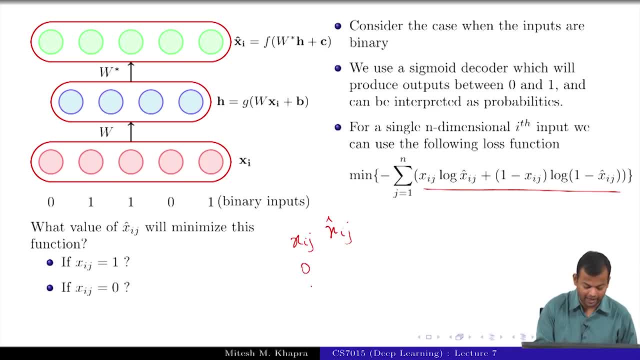 x hat i j is equal to x i j. right, So now x i j could take value 0 or 1. ok, and now x hat i j could take 0, 1 or 0, 1.. So you can see that for these two combinations, the value is going to be minimized only when. 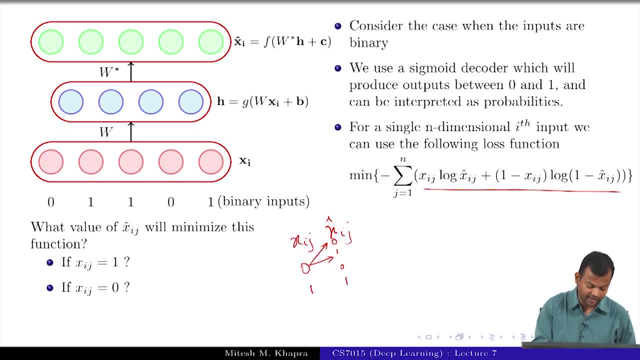 x hat i j is actually equal to x i j. that means if x hat, if x i j was 0, then x hat i j should also be 0, and similarly in this case also if x i j was 1, then the expression will be minimized only when x hat i j is equal to 1.. So let us see this right. So suppose 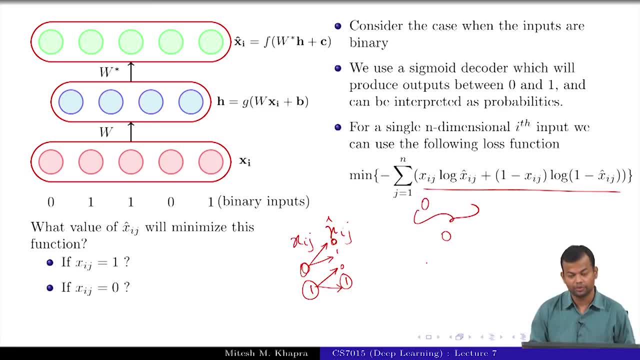 x i j was 0, that means this term is going to go to 0, but this term is going to remain. and now if your x hat i j was not equal to 0, then you will get some log of 1 minus x hat i j as the loss right. But if x hat i j was also 0, then you would get log of 1, which 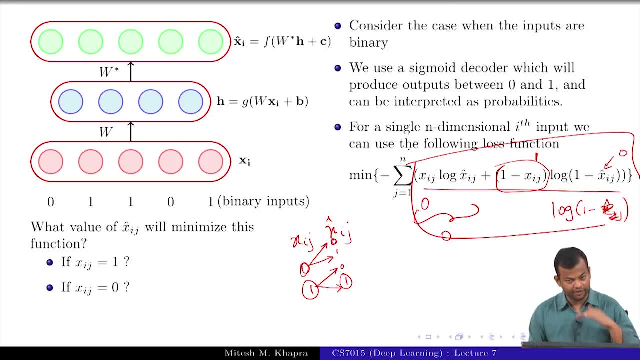 is 0.. So this whole expression would then evaluate to 0, which is the minimum possible value for this expression, right? So that means if x i j is 0, then this expression will be minimized only when x hat i j is also equal to 0.. 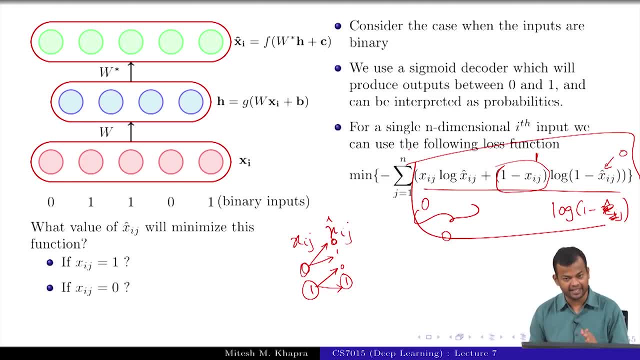 Similarly, if x hat i j, is sorry. if x i j is 1, then this 1 minus 1 will give you 0. So this term is going to disappear, but this term will remain, So this will just be log. 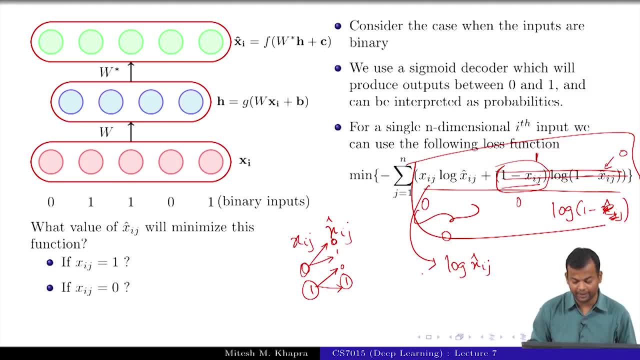 of x hat i j because x i j is equal to 1.. Now if x hat i j is also equal to 1, then this will become log of 1, which is 0. that means again, this expression will attain its minimum value when x hat i j is equal to x i j is equal to 1 right. 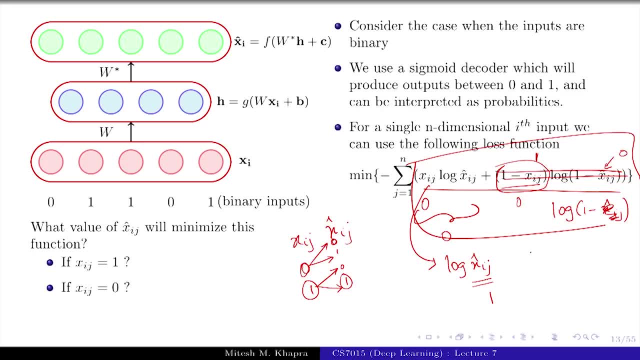 So this expression will attain its minimum value in two cases: when x i j is equal to x, hat i j is equal to 0, or when x i j is equal to x, hat i j is equal to 1.. So compactly I can say that this expression will attain its minimum when x i j is equal to x hat i. 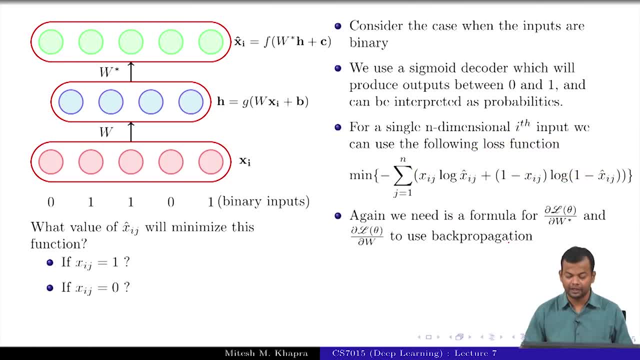 j. that is why this loss function makes sense. ok, Now again we have this problem that we want to use back propagation to train this network. and once again, for back propagation, we will need the following gradients: the gradients of the loss function with respect to w and. 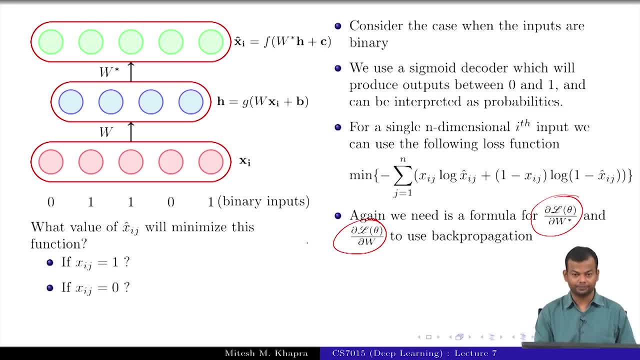 w star. ok, This is what we are going to need, and I am going to make the same argument again: that whatever hard work you had done in the back propagation lecture, you can just reuse all of it, because the only thing you are changing is this final loss function. So just need: 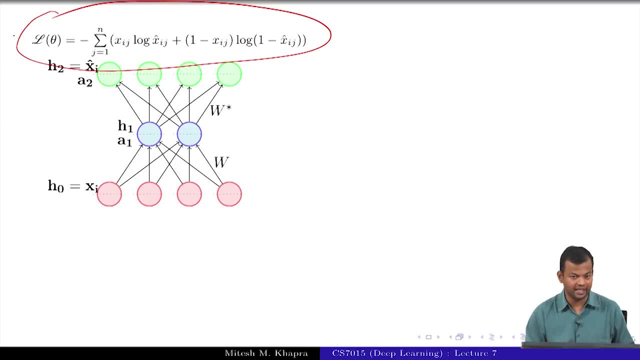 to compute the gradients with respect to this loss function, and everything else is going to remain the same right. So that is exactly what I am going to do on this slide. So, whatever is in the boxes Here, these two boxes, that is something that you have already computed, and now what I am. 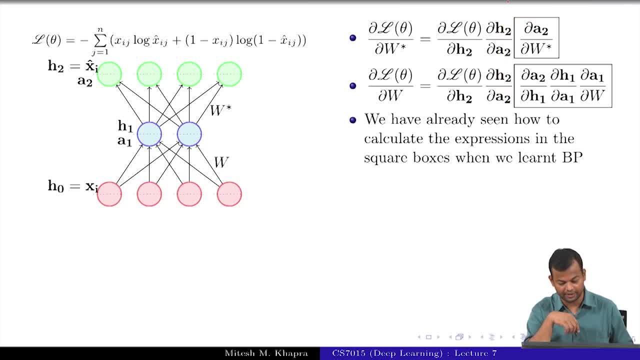 going to compute is the stuff which is outside the boxes. So let us look at that. So I am interested in computing this dou L theta by dou h 2. this is the derivative of a scalar quantity with respect to a vector, So it is going to be a vector and I am going to 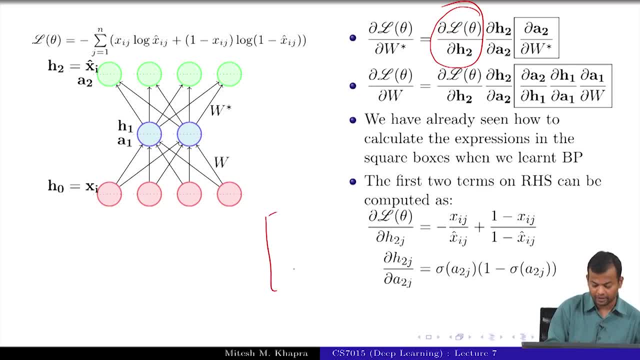 follow our usual recipe, which is h 2 is actually equal to h 2, 1.. So h 2ACE is h 2 x, H 2, h 2 up to h 2 N. So I am going to consider anyone of these guys. 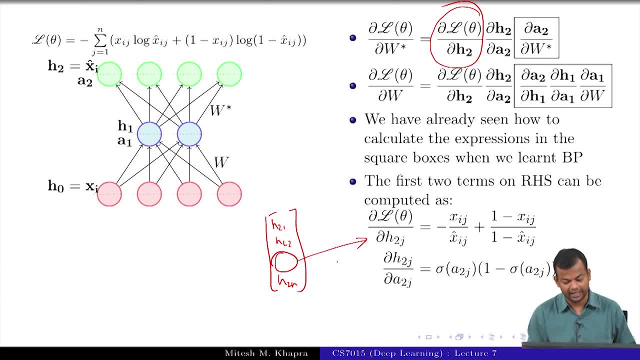 which is h 2 J. I am going to compute the derivative of the loss function with respect to this one entry and once I have that I am going to construct the entire gradient right. So now I will have this dou L theta by dou h 2 J right. 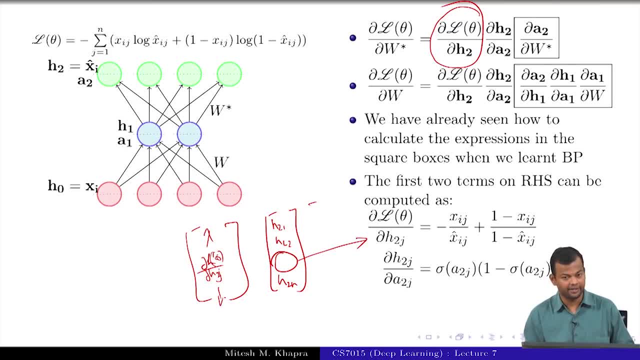 And once I have that expression, I am just going to generalize it to all the other entries in this vector. So let me sort out these data and I will come back in a minute. ok, So let us look at that expression first. ok, So now, if you look at, this actually does. 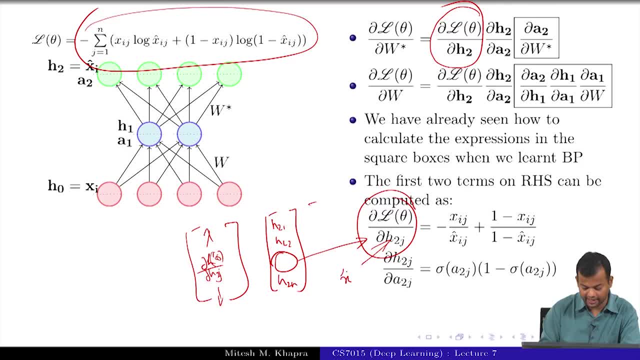 not have an h 2 j. right, but we know that h 2 j is the same as x hat j, or rather x hat i j. right for the ith input, it is going to be x hat i j because h 2 is equal to x hat. 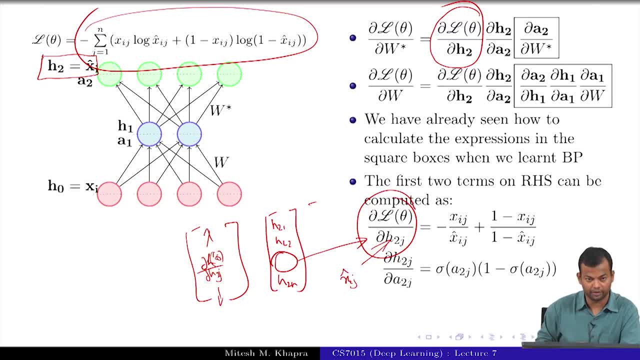 i. ok, You can just see that the top left corner of the slides. So h 2 is equal to x hat i. So this is nothing but dou L theta by dou x hat i j. So now I want to take the derivative. 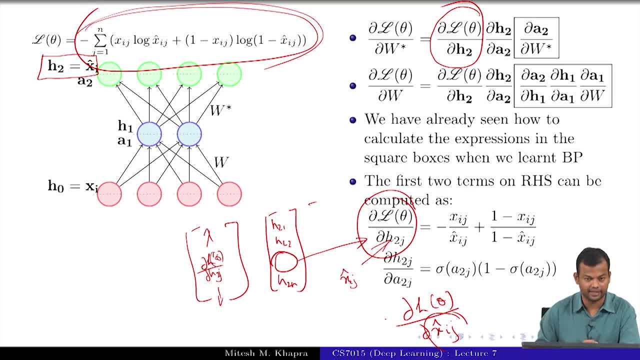 of this quantity with respect to one particular x, i, j, and remember that this quantity has a sum which is indexed over j, So j goes from 1 to n. I am looking at one particular j. So that means, if I expand this sum of all the j's possible, the derivative with respect. 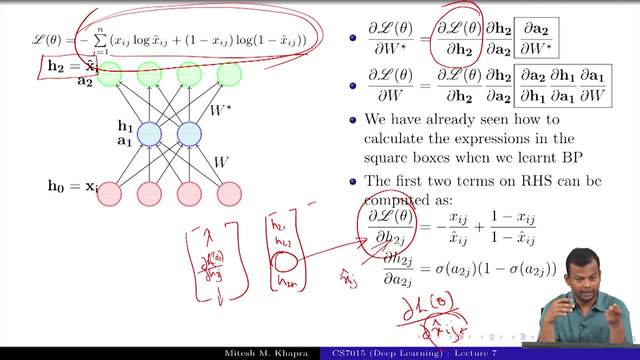 to all but 1 is going to be 0.. because they do not depend on this particular j. So if I am looking at j equal to 3, then the term which has x hat i, 1 is going to. the derivative of that term is going to be 0.. 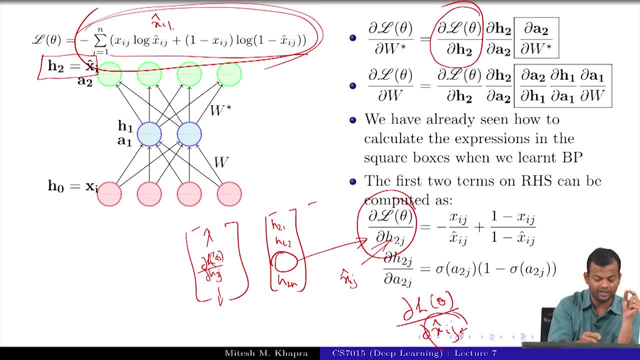 So of all these terms in the expression, only that term where j is equal to the j, which I am considering, is going to remain. ok, So that means only one term in the summation would remain, and for that one term. So let me just get rid of the summation, right? So 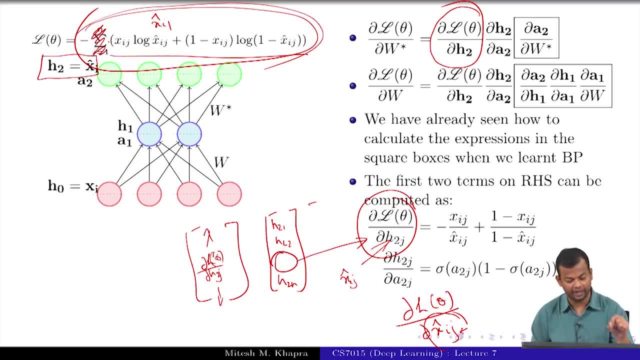 that means only one term in the summation would remain. I am trying to find the derivative of this quantity x, which has a lot of x i j's with respect to x i j. So now this is of the form a log x, So the derivative would be a over x, right? So that is exactly what. 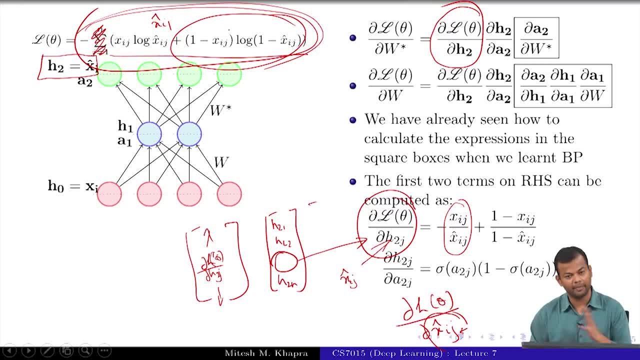 I have written here and similarly for the second guy. this is 1 minus a into log of 1 minus x. So the derivative is going to be 1 minus a over 1 minus x and of course there is this minus sign here which will then get adjusted approximately. 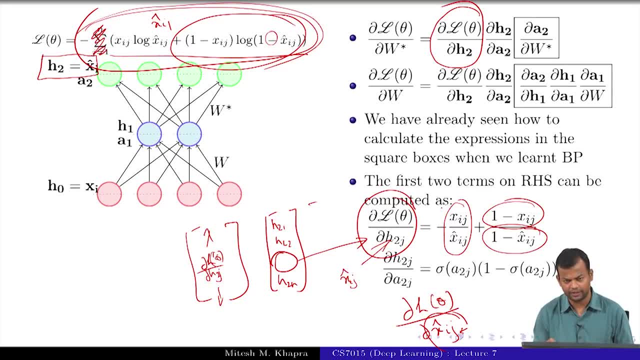 So that is how this expression has been completed. that is very straight forward. and now I also need the derivative of h 2 j with respect to a 2 j. So remember that h 2 is equal to sigmoid of a 2, which means it is just an element. wise sigmoid, right. So I just need to compute. 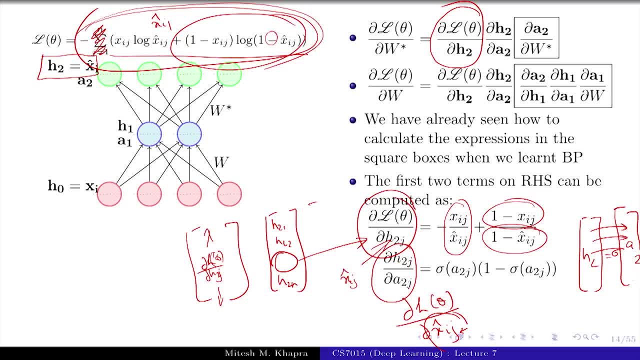 the derivative of the jth entry of h 2 with respect to the jth entry of a 2. all the other derivatives are going to be 0. Because they do not depend on that particular entry of a 2.. So now that is just going to. 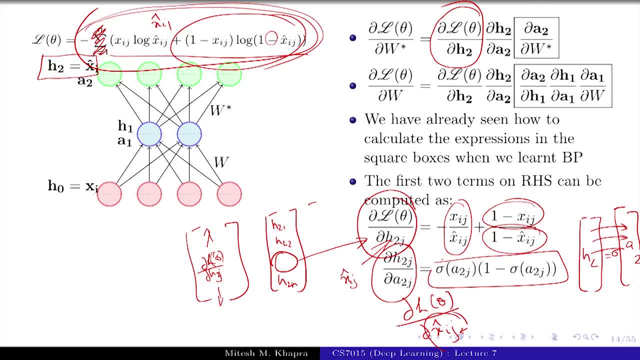 be sigmoid of a 2 into 1 minus sigmoid of a 2, right. So I have computed these two quantities. I can just plug it them back into our back propagation code. the rest of the code is going to remain the same and I have the gradients ready with me, right? And as I said once, I 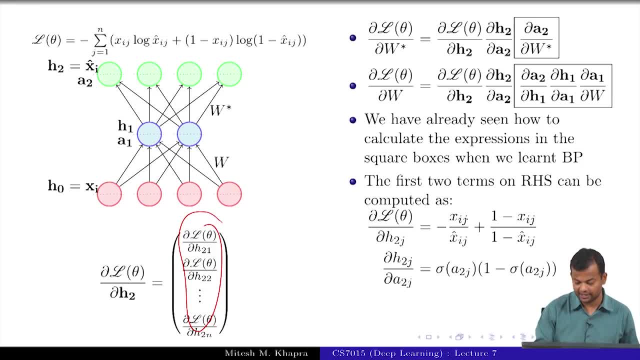 have this one guy. I can just extend it, I can just generalize it. So I just had these j's here right for h 2 j And I will just place the j by one, two up to n and I will get the same expression. ok, 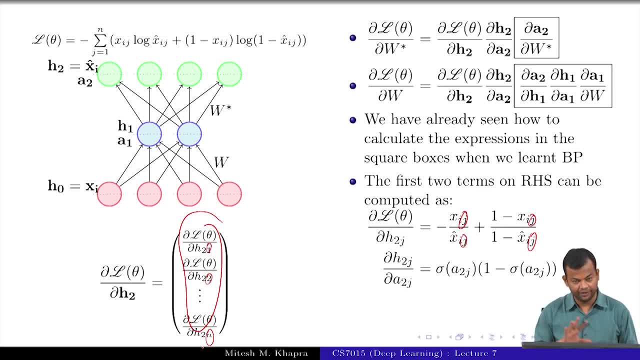 So that is the end of module I, where we introduced auto encoders. What we showed is that they are actually just like any other feed forward neural network, except that they have this spatial objective that they want to reconstruct the input And the reason they want to reconstruct. 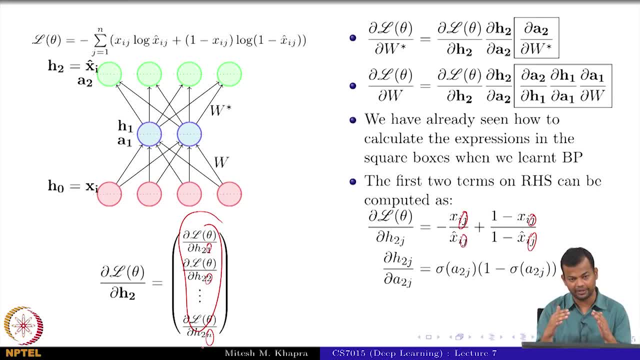 the input is they want to first create a bottleneck, which is this edge, hidden representation, and then try to reconstruct from their- And just as I gave you that compression analogy- that you have this 10 bits, you want to compress it to 4 bits and then reconstruct the entire input again. 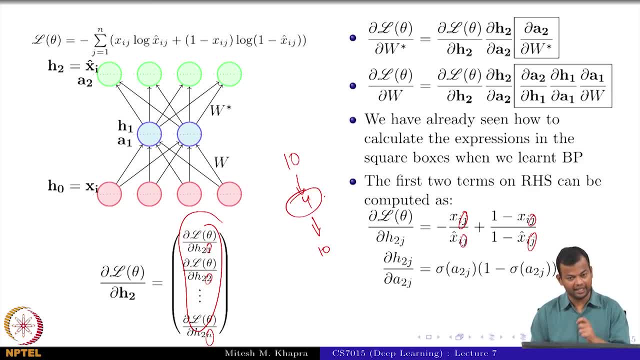 So this will happen only if these 4 bits capture everything that is required, or the most important characteristics of your original input, right, And then we could have a loss function which tries to capture the difference between my original input and my reconstructed input. 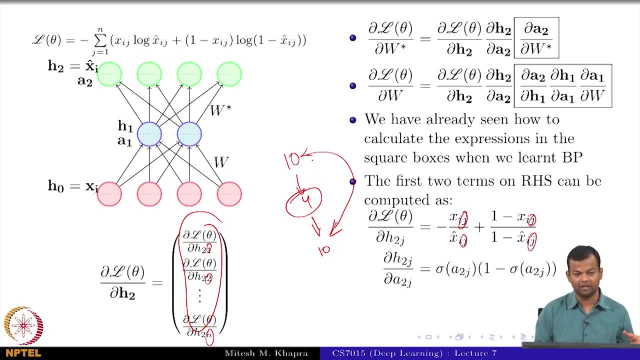 Now we argued that this loss function will be dependent on the nature of your input. So for the real inputs, it was straightforward: we just said that we can use the squared error loss function. For the binary inputs, we actually did something special. we said that we can actually use 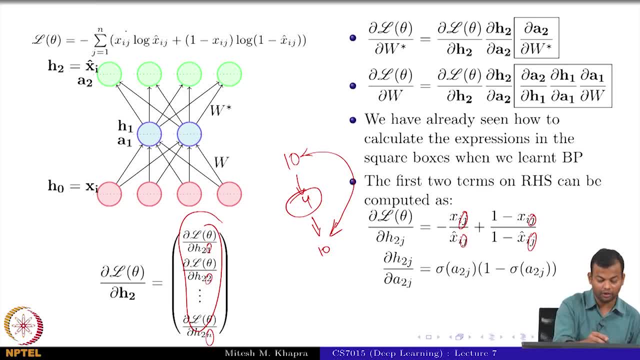 the cross entropy. And then we had this funny way of writing the cross entropy, which was this: x i into log of x hat and 1 minus x i into log of 1 minus x hat. and this gave you some intuition that that is the same as writing p log, pi log, or rather p 0 log, q 0 plus p 1 log, q 1.. 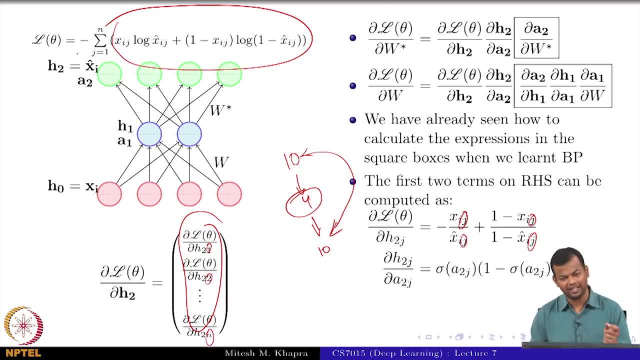 And I just gave you some explanation for doing that. You can go back and check on how do you write the cross entropy for Bernoulli random variables and you will see that this expression makes sense. And once we had this expression, computing the gradients was easy. 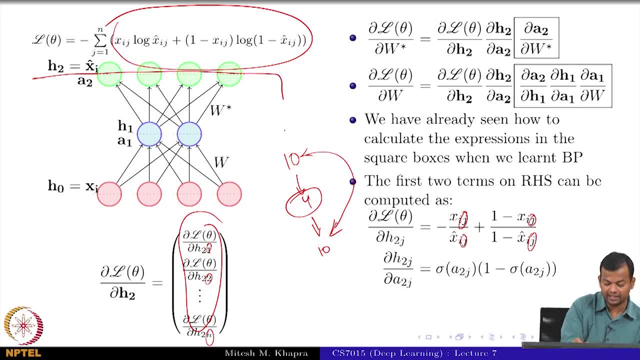 So the other thing that we relied on is that in the back propagation lecture we had taken care of everything up to this point, and in this lecture we have actually changed the loss function. So one loss function was the sum of squared loss errors, and the other loss function was 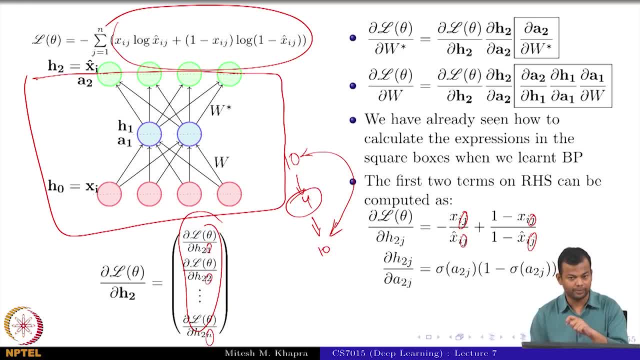 the sum of The sum of cross entropies, whereas in the back propagation lecture we are only dealt with cross entropy. But the case that we made is that, since you have this chain and all you have done is change the last function in the chain, right, you have changed this l function, all the other. 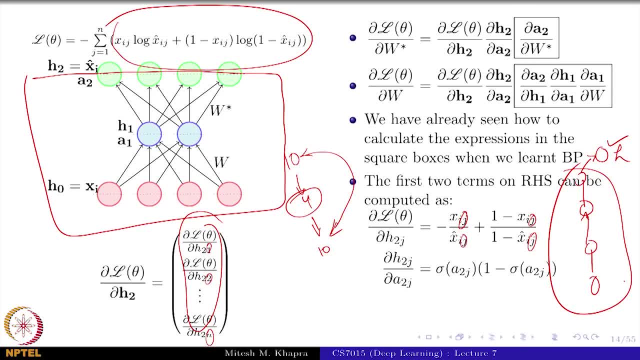 functions you have not changed. You can just reuse the computations from these. or you can just reuse the code that you had written for these in the back propagation assignment, and you just need to change this last guy to adjust for the change in the output layer or the change in the loss layer. ok, 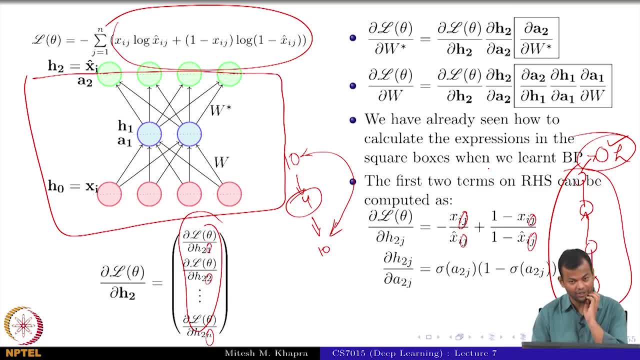 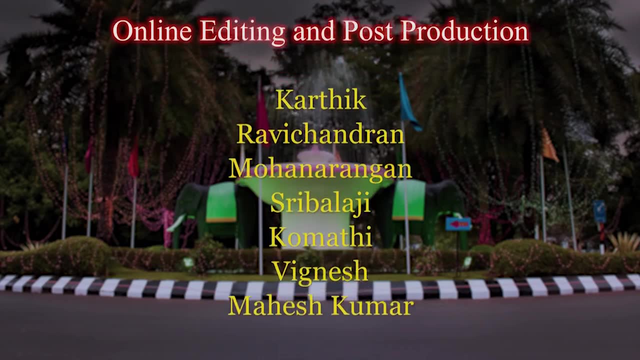 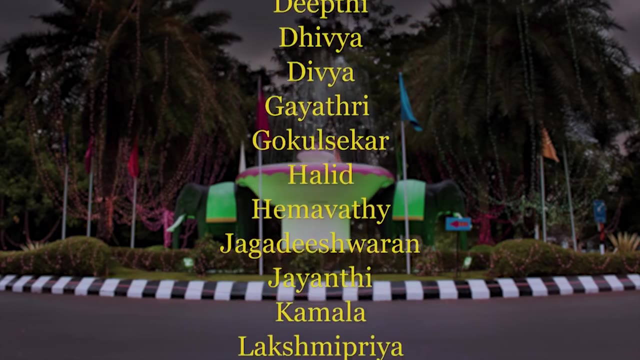 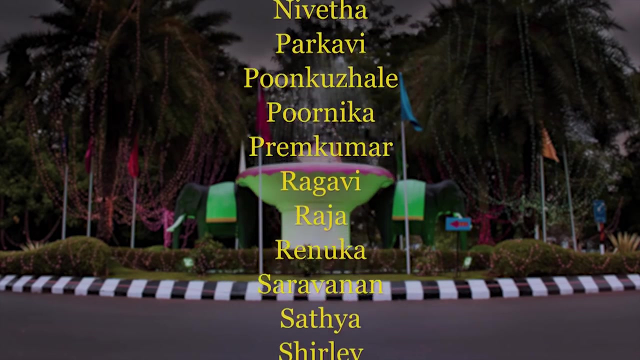 So with that we will end the introduction to autoencoders. where we have done, we have actually covered how to train an autoencoder using back propagation. ok, So that is where we will end, Thank you.